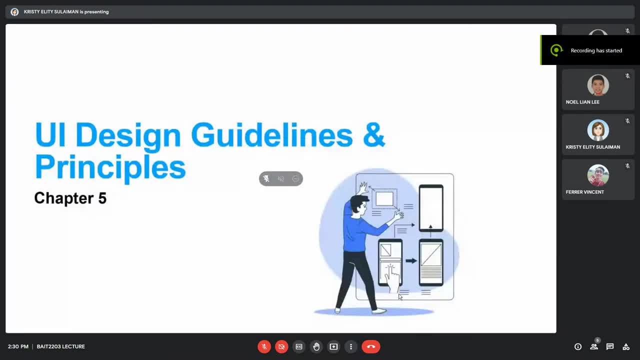 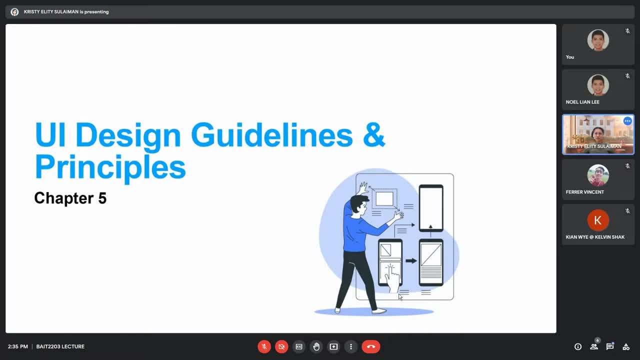 cost it's in. yeah, so for this course, HCI, the medium test will be online, which is open book test. it will be conducted during lecture, okay, so means on Wednesday at this time in week 8. I will put announcement in the classroom later on, so it should be. 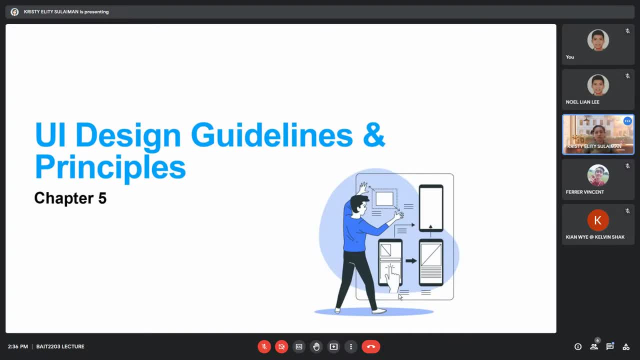 9 of March. 9 of March, okay, during lecture time. yeah, yeah, I will post an announcement in the classroom. so the the format, the moment of the. the format of the test. it's because it's open test it's. it will be like similar to okay. so the the format, the moment of the test. it's because it's open. 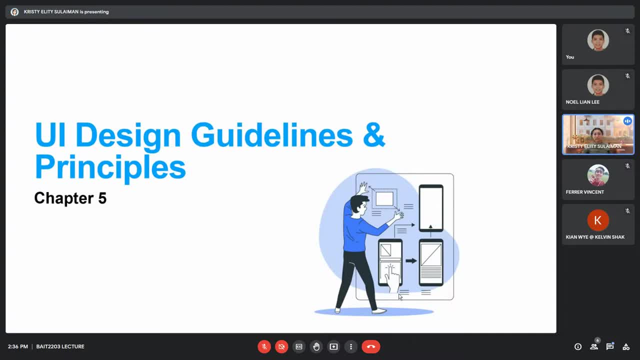 you given a scenario and you will need to discuss on the scenario and give your own opinion based on the theories and the concept that have learned from chapter 1 and 25. okay, so there will be only one question, one question with one scenario, and you will have a question 1a and Christian Monday and the total mark. 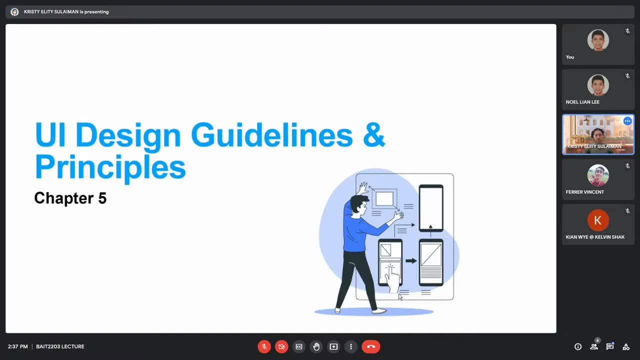 will be 30 months. okay, 30 months. so that's the actual mark for the meet and test. the assignment is 70- 70 months. so for your coursework you will have meet and test 30 months. uh, your project, your assignment is 70 months. total is 100- okay. 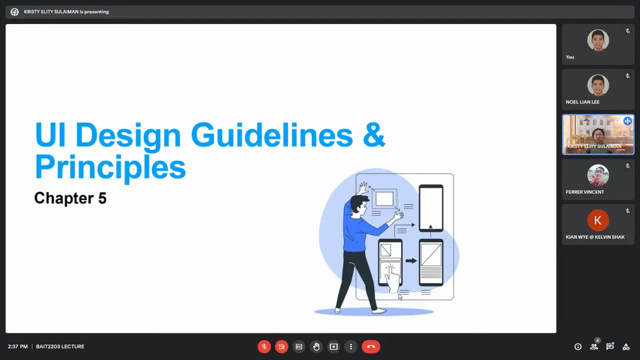 so, uh, i repeat, for the format, for the format you have, we have one question, um, it's a scenario. you're given a scenario, um, maybe regarding uh development of an app, development of uh an application, and then you will answer question based on the scenario that is given. 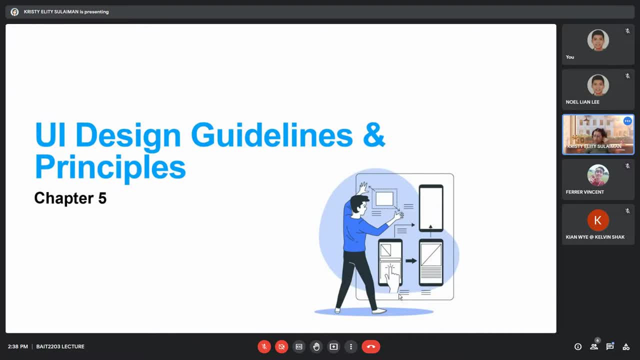 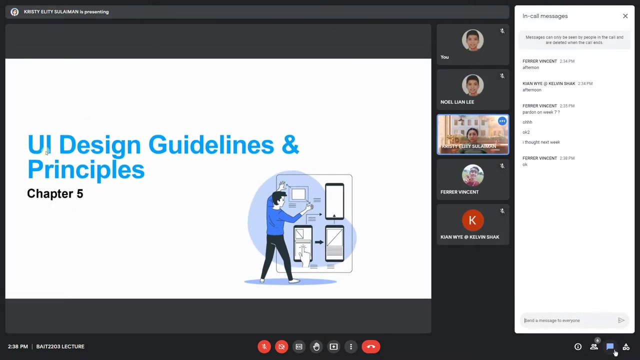 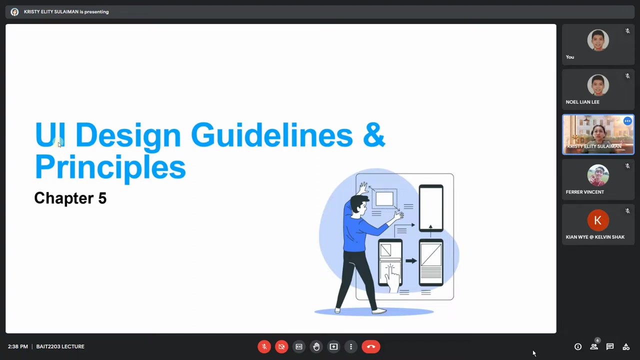 okay, so, yeah about that. okay and okay. so now we this week uh start on discussing chapter five. uh, for this, for today, chapter five. so we will now look at the ui design guidelines and principles. okay, so i have. i hope you have made progress for your project. okay, i hope you have made progress for your project. um, please do. 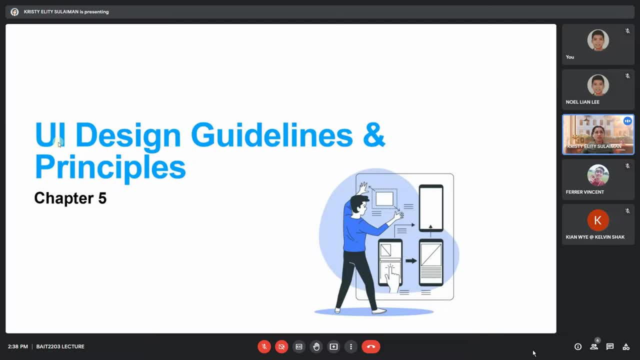 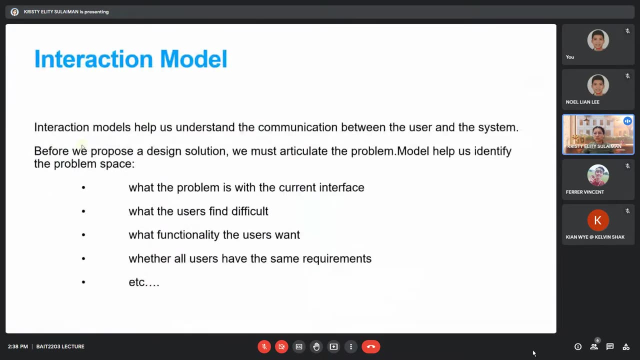 all the tasks that you have not completed in the previous weeks. right, so this is chapter five. we will discuss on the guidelines and principles for user interface design. okay, so first we want to understand what is interaction model. okay, so interaction model here it uh will help us to. 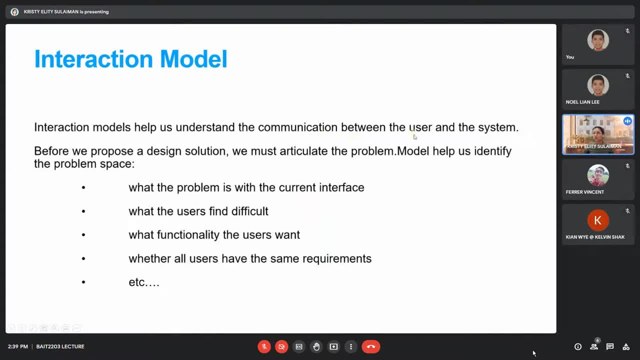 understand communication between the user and the system. so basically we want to have this interaction model where we will understand the communication of 2s between user and the system. so before we propose a design solution you want, we must first know the problem right. so in your 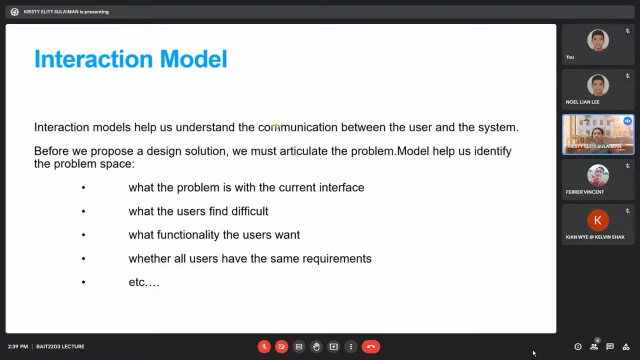 when you describe your persona at the first, at the earlier stage, we have look at the problems that your system want to look into or your system want to solve, right. so this interaction model will help us to identify the problem space. so we look at what is the what? 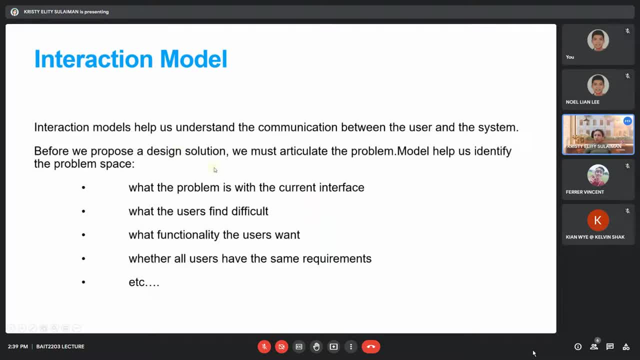 are the problem with the current interface, if any, and then what the users find difficult when they're using the current system and what are the functionality that the users want. okay, so this is one i think it's familiar to you, you already, when you you already do this uh problem segment in your 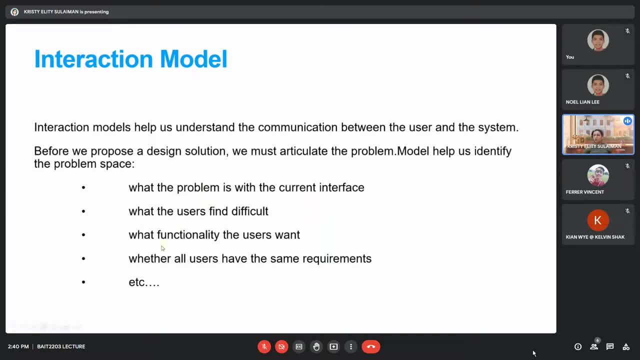 when you do your persona explanation and whether all users have the same requirements. okay, so, depending on your, depending on your app, depending on your system, does all users really want the same requirement? so, depending on if your user are students, you refer to students requirement, or user are adults, so you refer to adults requirement. okay, so for this lecture, we will. 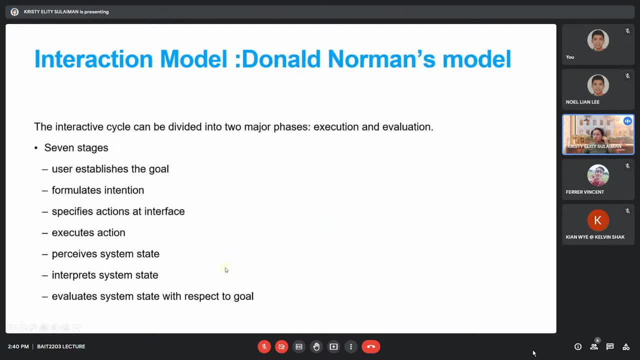 look at interaction model by donald norman's model. okay, so the interactive cycle can be divided into two major phases. so we have the execution and evaluation. the interactive cycle can be divided into two major faces, so we have the execution and evaluation phase. so we have the execution and evaluation. 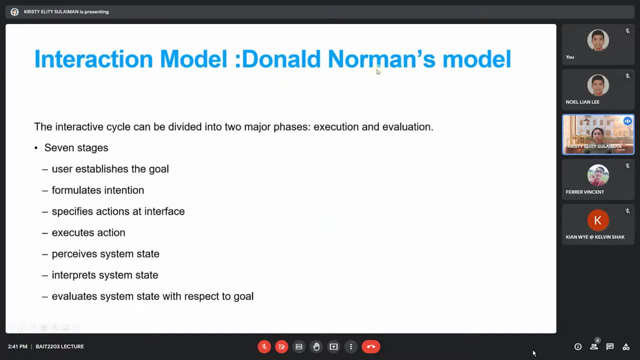 For this Donal Norman's model, we have seven stages. We have: user establishes the call and then formulate the intention and then specifies the actions at the interface and then execute the action, perceive system state and then it interprets the system state. 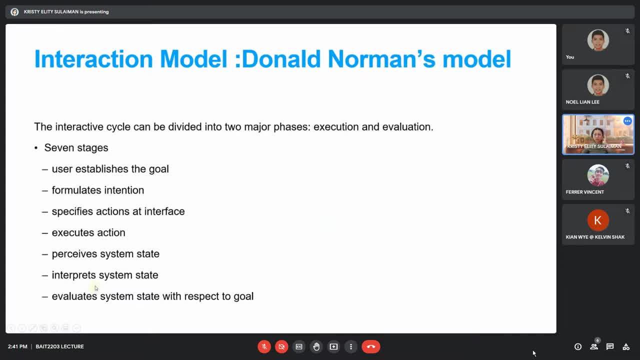 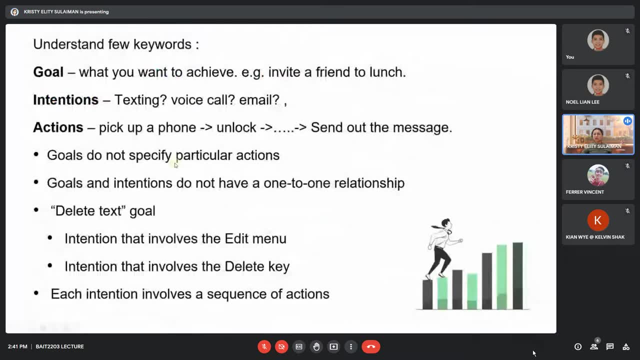 and the last one is evaluating system state with respect to the goal previously Before we proceed to discuss on the seven steps in the Donal Norman model. so you need to understand what are these few keywords. We have the first one: goal, intention and action. 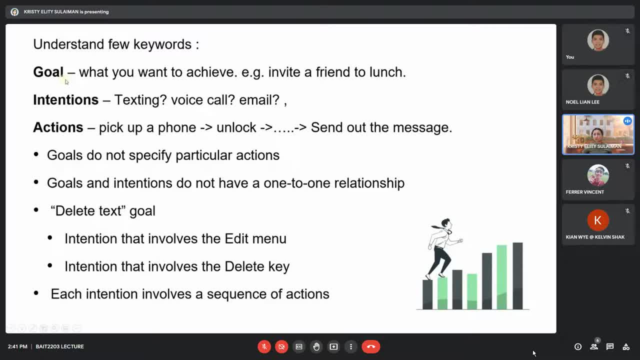 Goal is what you want to achieve. Example here: you want to invite a friend. You want to invite your friend to lunch. It's your goal. you want to invite your friend to lunch. Then, after you decide what is your goal, the goal is to invite your friend to the lunch. 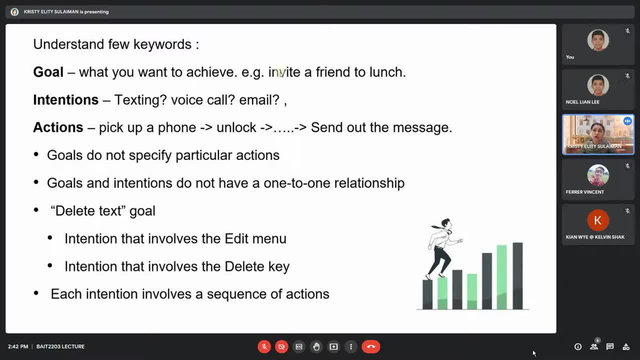 The intention here is where you think of various method on how to invite your friends to lunch. Maybe you text them, you use voice call, or maybe you email them. Okay, What types of intentions? So, after you decided on your, you pick one intention. 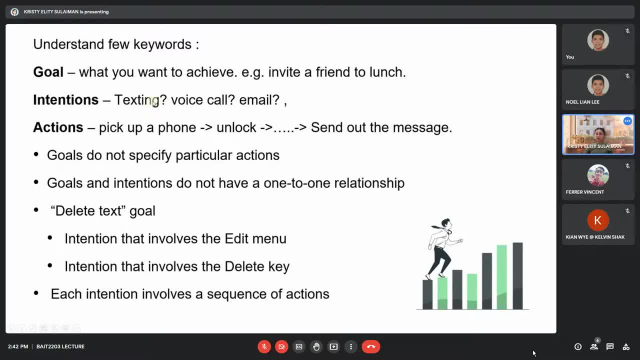 So here, for example, you pick texting right. So after you decided to text them, you will go to the next part, which is action. Okay, So you pick up your phone, you unlock your phone and then you open the messaging app. 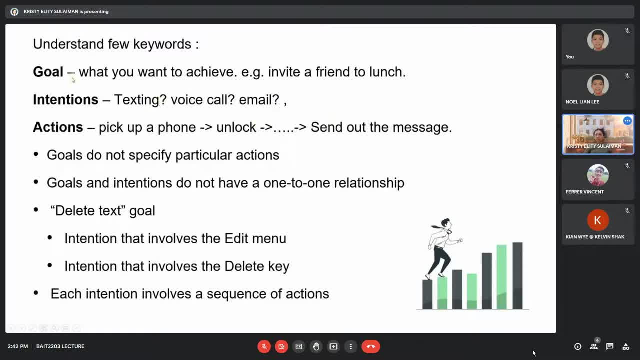 and then you send out the message: Okay, So these are the three keywords that you need to understand, And then you push it to discuss further into the normal model. the normal model, Yes, So for these goals it does not specify particular action. 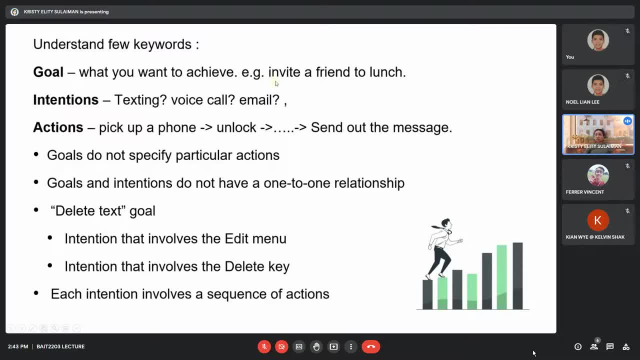 You just want to invite your friend to lunch, But you don't specify how to do this, Right? So goal is very straightforward, Like it's fixed. You want to invite your friend to lunch, That's it, Okay. So goal and intention do not have one-to-one interaction. 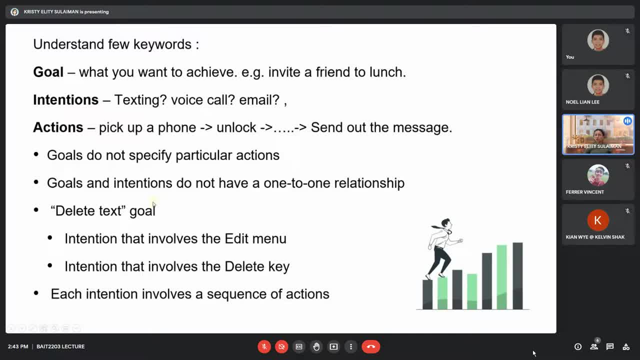 relationship. so your goal can can be one, but your intention can remain right. so let's say here: your another example is that your goal is to delete the text. okay, so intention, if you can, intention can have two. yeah, you can involve, you can get the text, you can have the delete function from. 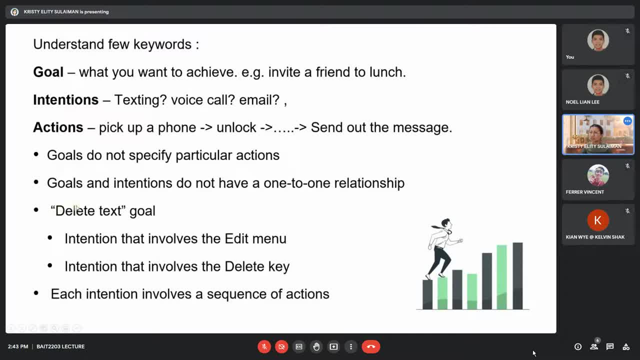 the edit menu or you can do this call. you can achieve this call by, uh, just press on your delete key on your keyboard. okay, so that's that. that's that's what me with this. do not have a one-to-one relationship. okay, so you can have one goal, but you can have main intention. okay, so every intention. 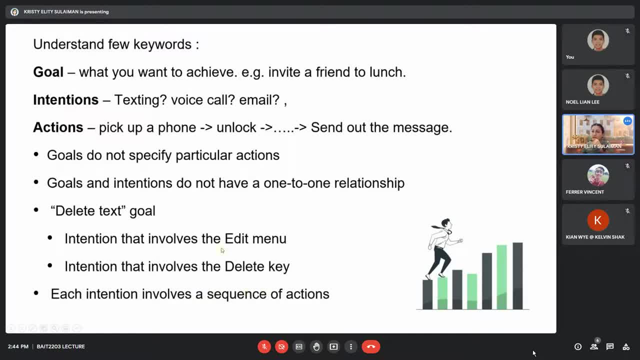 will involve a sequence of action, right, uh, if you use it, we know, so you need to cover your cursor to the edit menu and then you find the pattern right and also, um, similar to goes to this situation here, where the action is: you've got a phone, you unlock, right, so action can be sequence. 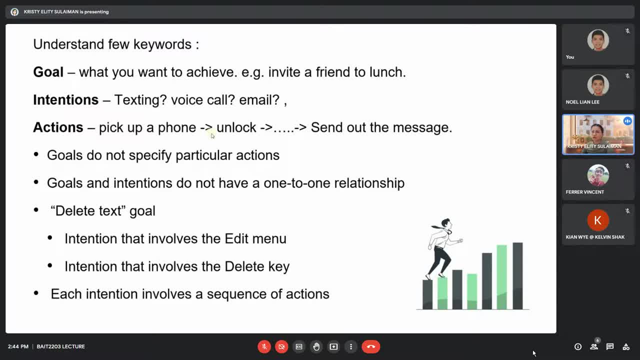 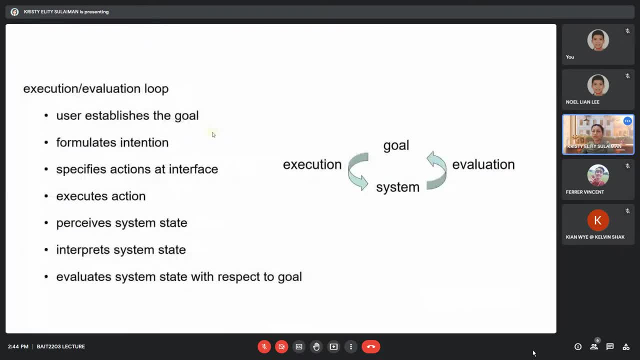 of um sequence of actions, sequence of activity, yeah, so let's now look at the first step in the normal model. so we have execution and evaluation. uh, all these are seven, seven steps. okay, so the normal model actually refers to this um figure here. so first we will have the goal. 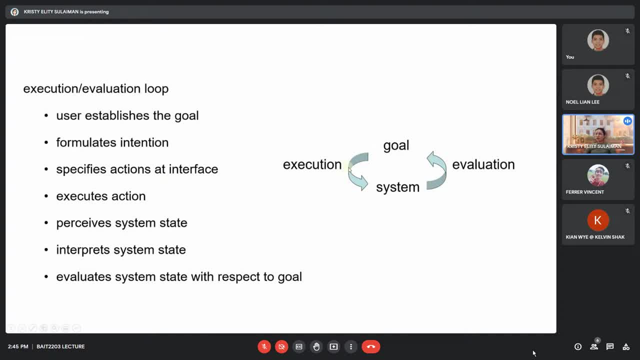 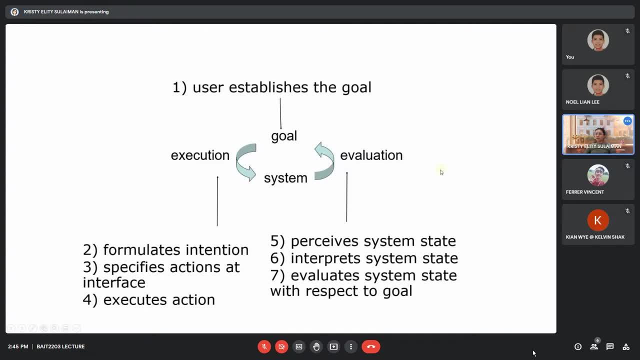 and then we'll have the execution. uh, and then we go to the system and we have the evaluation. so here is where the seven steps are um scattered. okay, so you have number one: user establishes the call and then you execute it. you can formulate the intention and then you specify actions at the systems interface and you execute the actions and then. 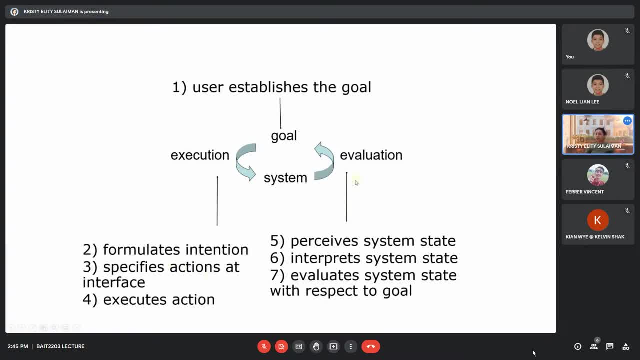 you go to evaluation phase whereby you perceive the system state, the current, the current state of the system after you have done the action. and then you interpret the system state after you, uh, do the action. and number seven, you evaluate the system step with respect to go okay, so you. 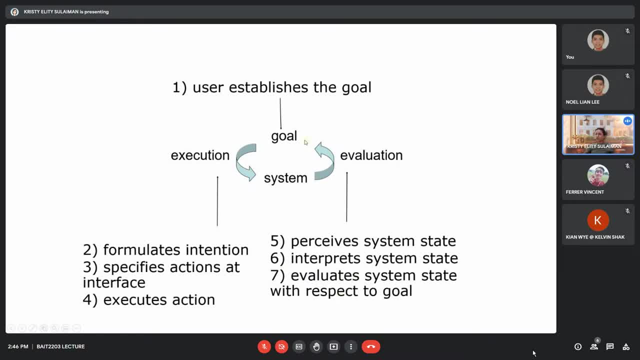 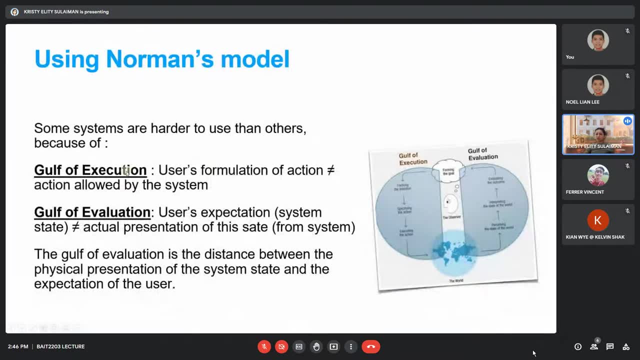 evaluate the system by referring back to your code. okay, so, when we are using this normans model, uh, we have these two go, okay, called of execution and we call of evaluation. so this is, um, this is, uh, just a theory or a concept whereby, uh, with this, uh two. 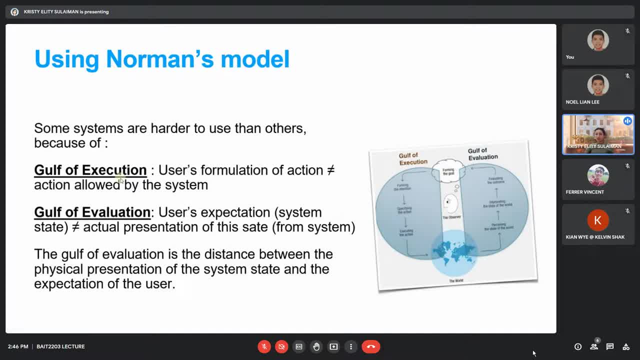 with these two girls. um, it differentiate between systems. some system can be harder to use and some system can be easy to use. okay, so then, like, for example, you have the goal of exhibition. so the user formulation of action does not necessarily be the same what the action allowed by the system. 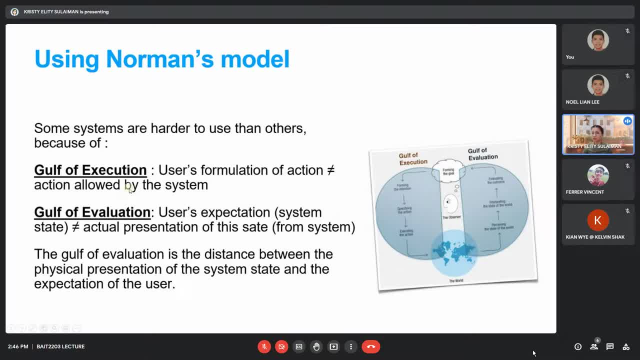 okay, for example, like the example just now, when you want to make your friend to lunch, right, and then your action would be: um, sending, texting. your intention is texting, and the new action is: you open your. you open your mobile phone. uh, so maybe let's say, for example, like: 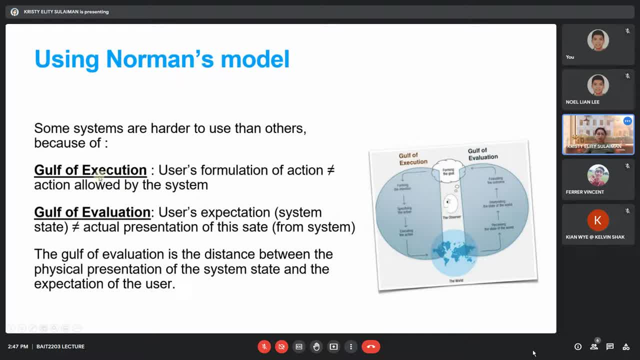 uh, if you are, you have this goal of execution. maybe your phone, mobile phone, you don't have any texting, messaging, texting app, for example. that's an example. so everything that you think of, that you want, your intention and your accumulation of action in your mind does not always uh allowed by. 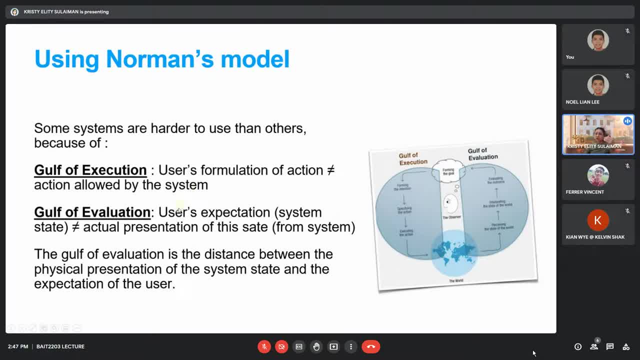 the system. okay, so uh, the next one is the golf of evolution. so the user's expectation, our own expectation, um, of the system state, is not always the same with the actual presentation of this, the system of his state get. so our expectation not necessarily always the same with what we have for the 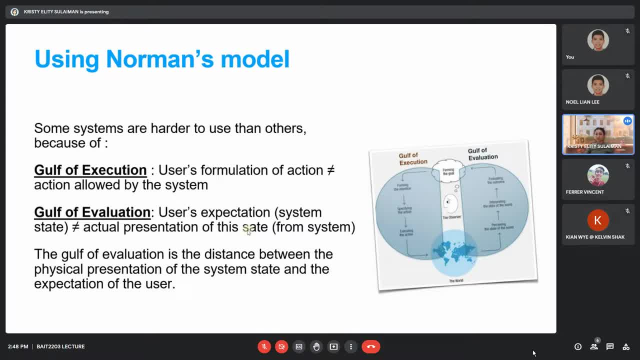 it will not always be presented by the system. so the goal of evolution it's a distance between the physical presentation of the system state and the expectation of the user. so the user expects something else, and then the system give you something else, right? so that's the that's. 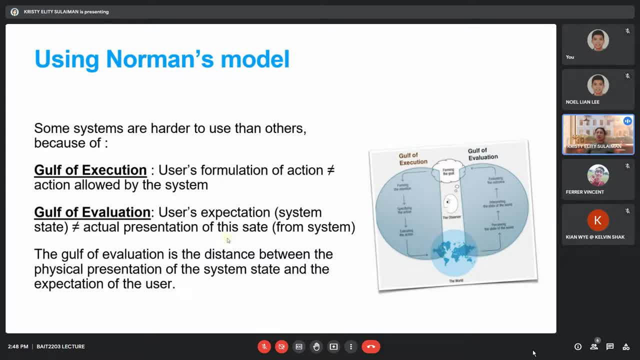 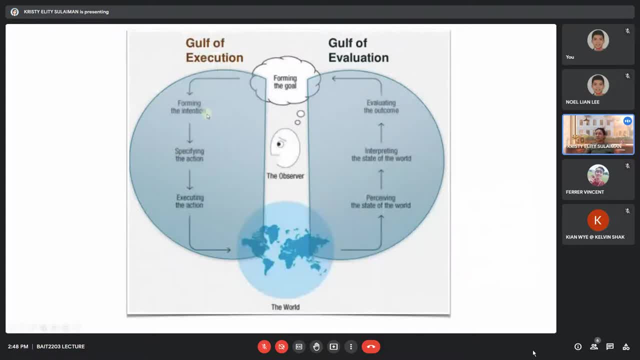 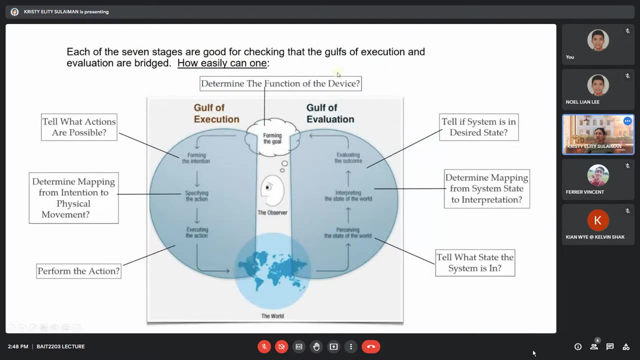 explanation for this too. so we can say: these are the challenge challenges of this model. so here it's showing you the curve of execution again from the normal models, and the correlation for each of the seven stages are good for checking them. the curve of execution and evolution are: 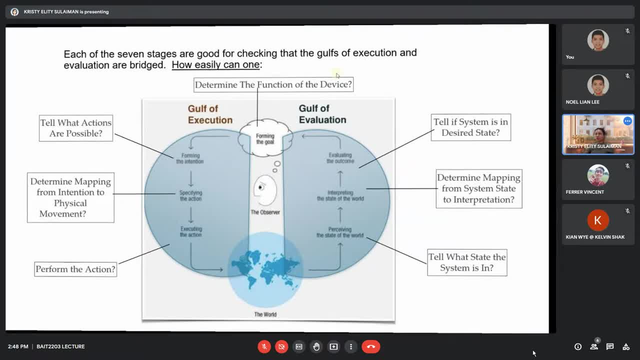 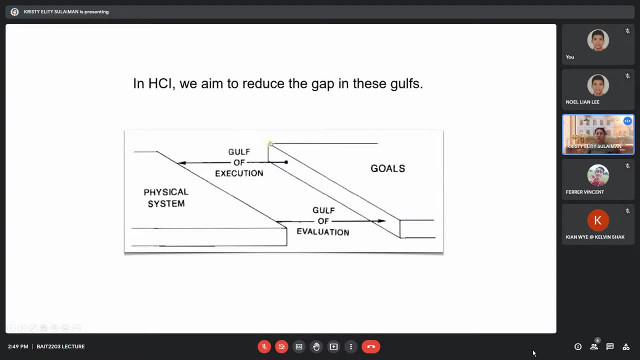 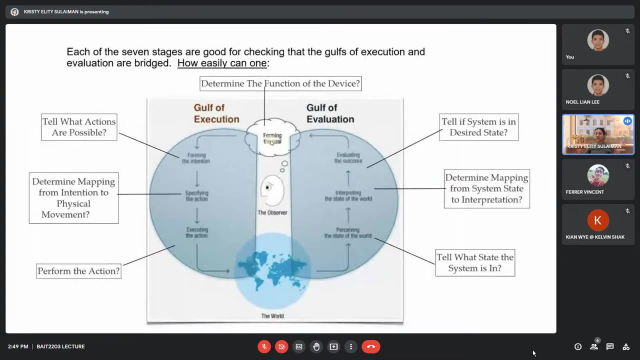 bridge every training to say we want to reduce the gaps between this go, can you? we want to at least reduce you the gap between the golf um in hci. okay. so here example like how easily can one determine the function of the device and then, uh, tell what actions are possible? 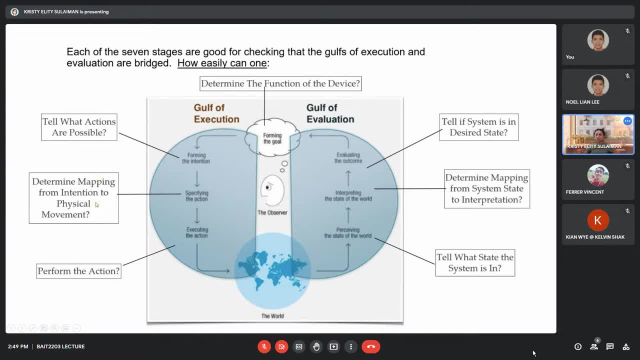 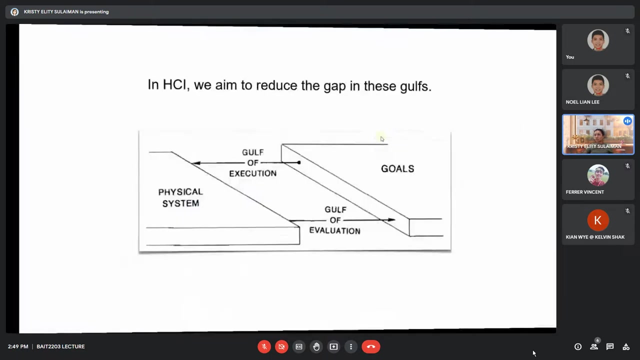 determine the mapping from intention to physical movement. you perform the action and then tell what states, what stack the system is in and determining the determining mapping from system set of interpretation to interpretation and tell if the system is in decided step. so it's hci, uh, aim to. 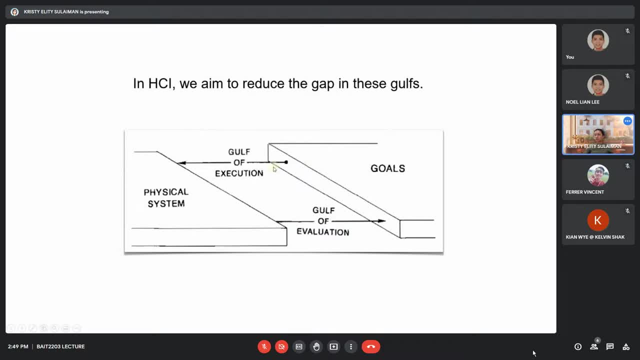 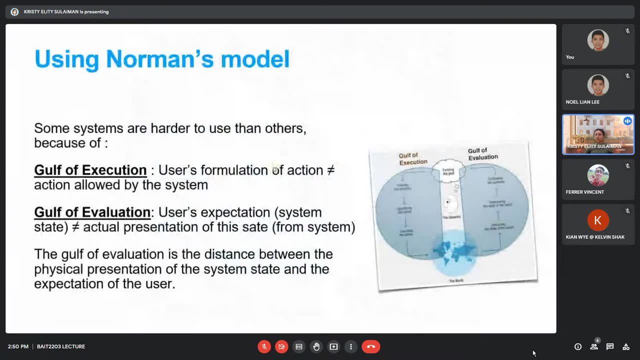 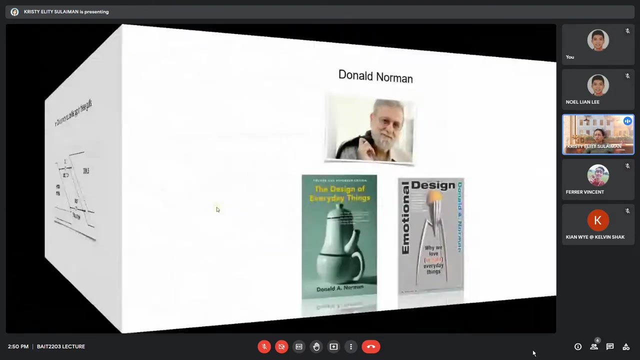 reduce the gap between these goals. okay, so at least, um, we want to make sure that our design will. um, it will remove this goal. okay, so your exchange should be allowed by the system. your expectation should be the same as the actual presentation of your system. okay, so the next part. also, this is a book of this expert. in hci he has these two books. 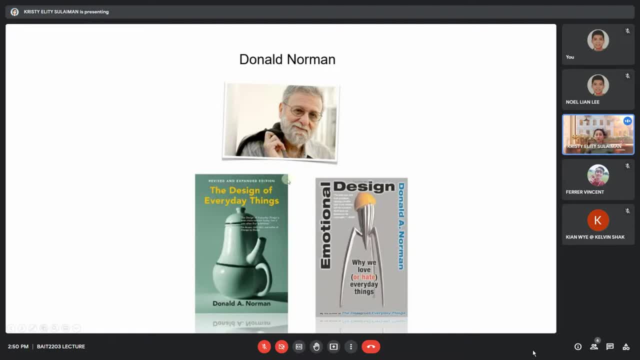 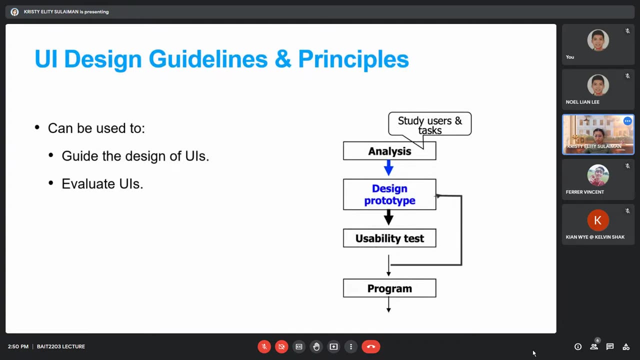 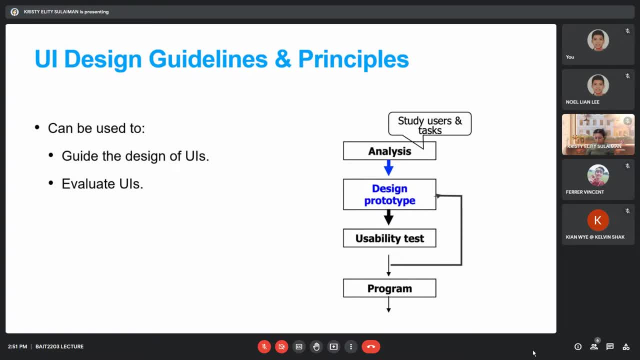 you, Thank you. So now we will look at some guidelines and principles for UI design. So we are now at design prototype, this part. We already studied the uses and the tasks And now you are doing practical. We have done the storyboard, okay. 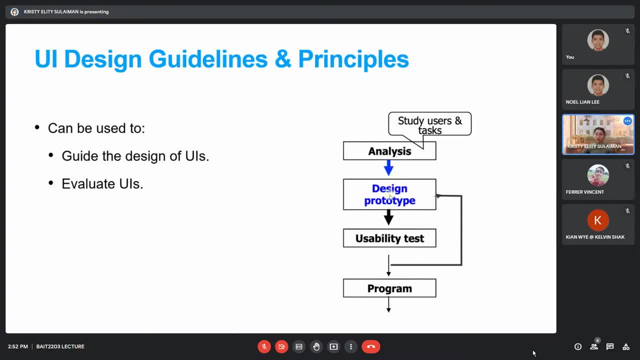 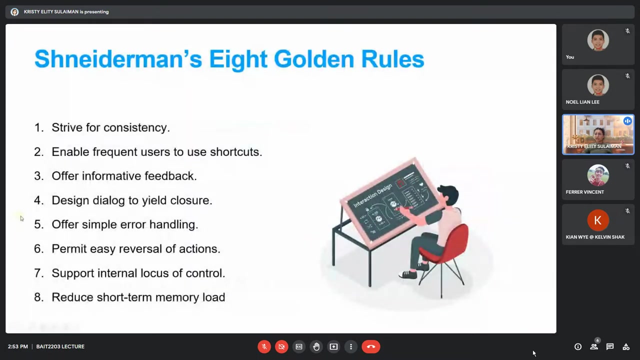 We have done the storyboard and you should have drafting your storyboard, So we will look at some guidelines to design Your UI and how to evaluate your UI. Okay, and then we have another golden rule for this UI design. We will look at each one of these for how to achieve a good UI design. 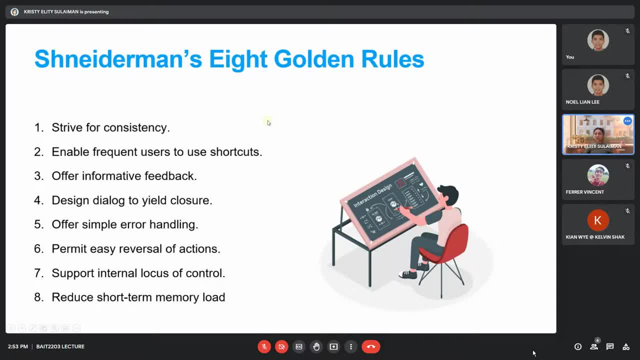 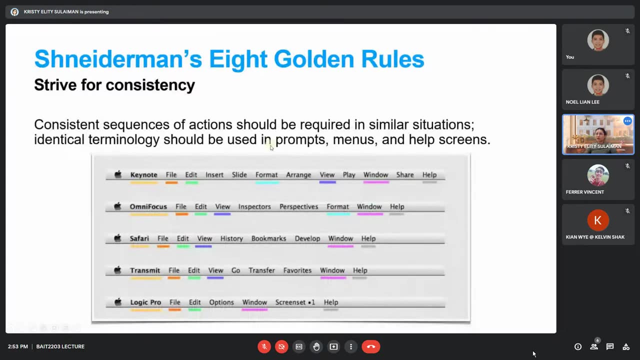 Okay, Basically the ideas on how to achieve a good representation of UI. Okay, so we look at all these eight golden rules. Okay, so we go to the first one. So strive for consistency. So when you design your system, you should apply this consistency in your design. 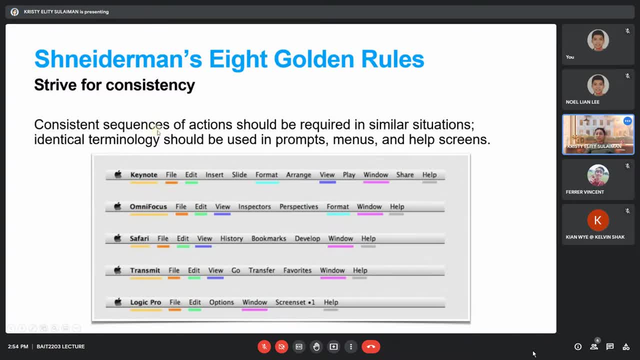 Like, for example, your action should be In a similar situation, like when you have a button. when you have a button login. So let's say you use the font Times New Roman, So you go to either page. your button or your other button should also use the same font type, for example, 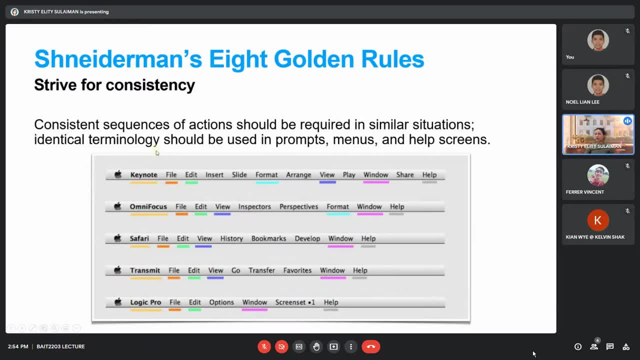 Okay, so you should have identical terminology that you use in promp menus and help screens. Okay, so, meaning to say you have a consistent. So let's take this an example. So like this one right, This example of menu button for several types of application in Mac OS. 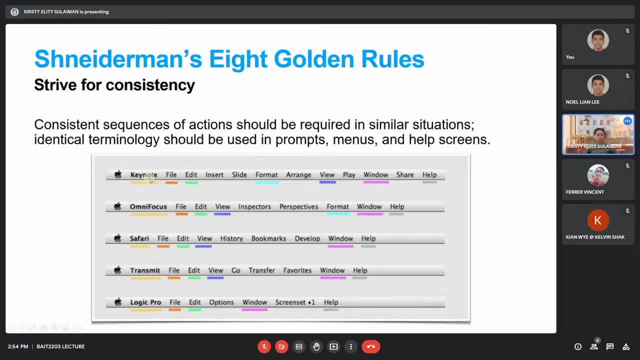 So this is for Keynote, So this is for Keynote. And then another app used in Mac OS Safari: Transcript Energy Pro. So if you notice, Okay, Okay, Okay, Okay. So if you notice the placement of the menu, the sub-menu are all at the similar position, right? 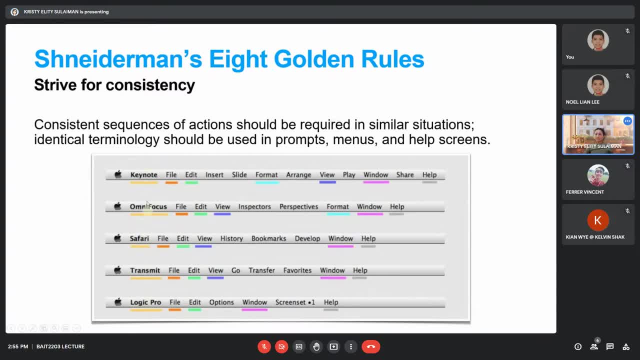 So you have the name of the app, the name of the software, and then file will always be at the most left side of the screen File, and then you have edit, the second one, And then you have view. Okay, So maybe here, because the rest doesn't have format, it is put at the end. 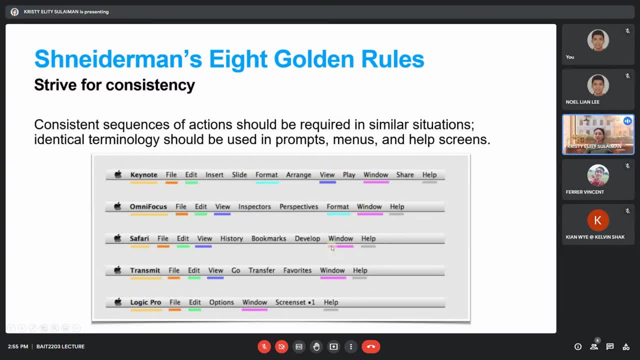 And then window always at the end, So that when you use your system they have this like, they have this like from the experience. or you open Keynote, the window is here at the end And then you open Safari, you will have this. 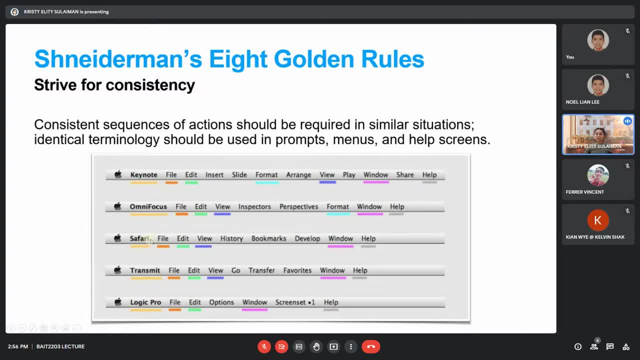 And then you put your windows here And then in Safari you will also put your Schritt Where you will believe that the software will also present window at the end. Okay, So let's say, for example: like it doesn't happen that way: 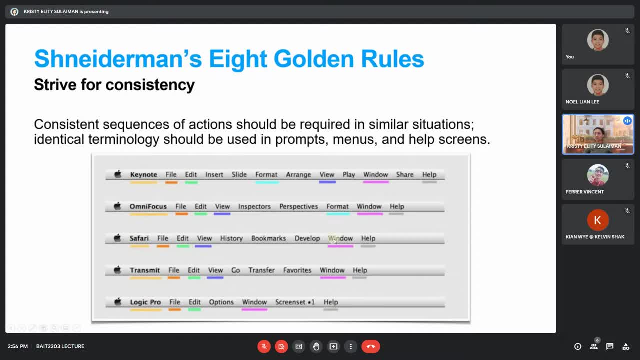 Like Safari, did not put this window here. Let's say it's under file, for example. So user can be frustrated because of that, because, like the other software is over here, but why the In this software it's not positioned at the same way? 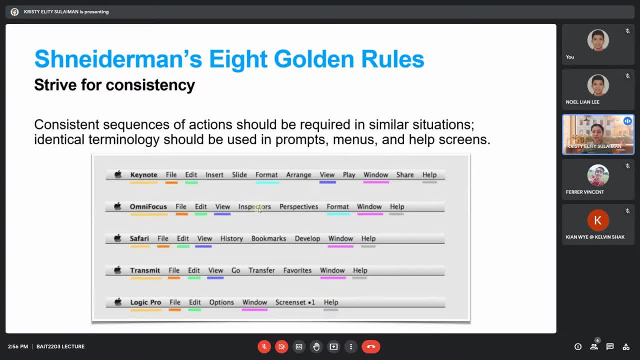 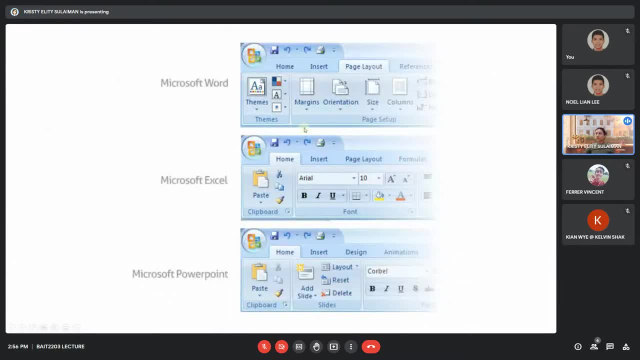 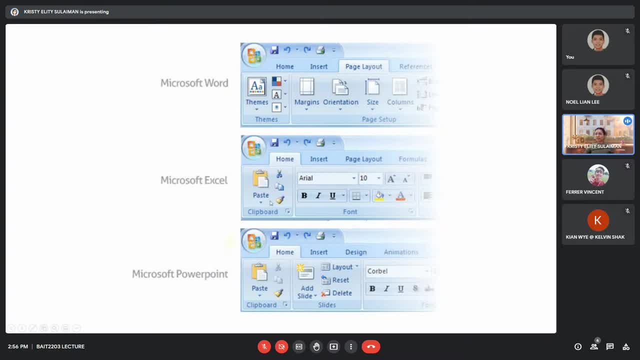 microsoft office for word, excel and powerpoint, which one are the biggest version and the municipal english one, microsoft 20, 20, 2019. yeah, so this one is the previous interface of office, so if you notice, every everything has a similar view. okay, so that it has its own identity. other than identity, it also helps users. 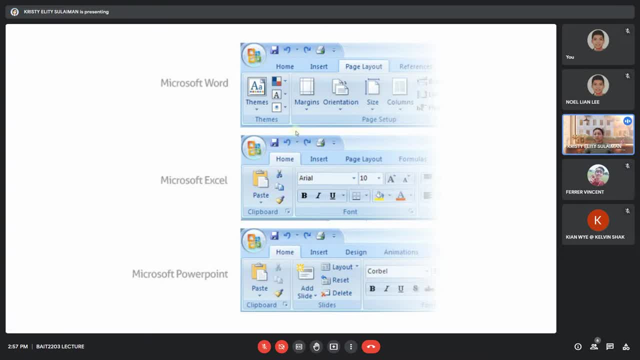 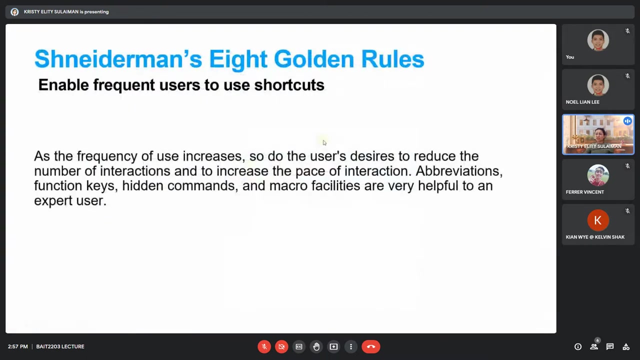 to like to manage, uh, the software that they are using, like they know where to go, so home is the same place, right insert also at the same place. so it helps user to use their experience to apply it to when they use a similar software. okay, so next we have the second rules. enable frequency, enable frequent users to use 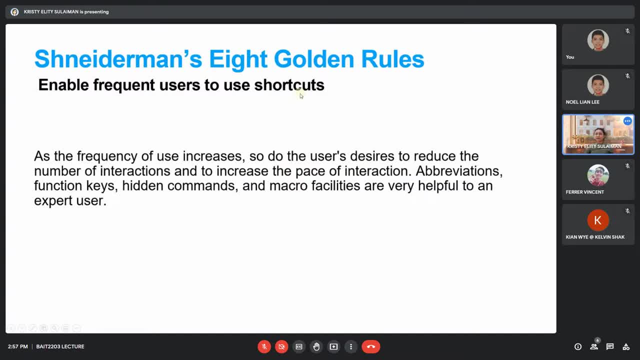 shortcut, okay, so shortcut, uh, here, when you, when you design your system, um, the user, like they, they tend to use shortcuts so that they can do their work faster. so, as the frequency of this increases, so to the user's desire to reduce the number of interaction and increase the fast of interaction, so they, they want to like, uh, have us some sort of shortcut. 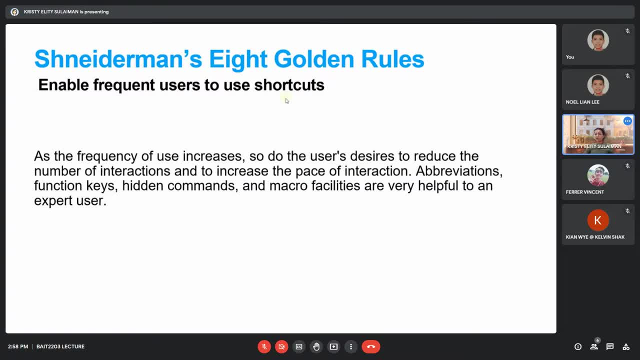 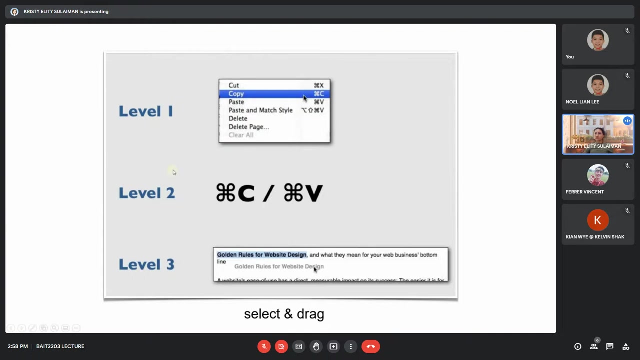 so that they can do their work faster. okay, so you can use abbreviation, you can use function keys, you can use a hidden commands and also macro facilities. yeah, but this one are more to more for, uh, expert user, all right, and then, uh, this is showing you, this is showing you the levels of shortcuts. so, level one: you can go to file and then you just 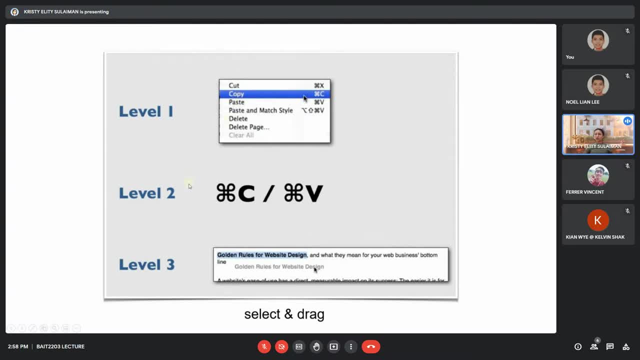 click on copy, level two of our shortcut. you can use control c, control v, so this one is for os. okay, then for mac os. then level three: you can use select and drag. okay, so in mac os you can do this, you can. you can select the text from any website and you can drag it and you can put it in. 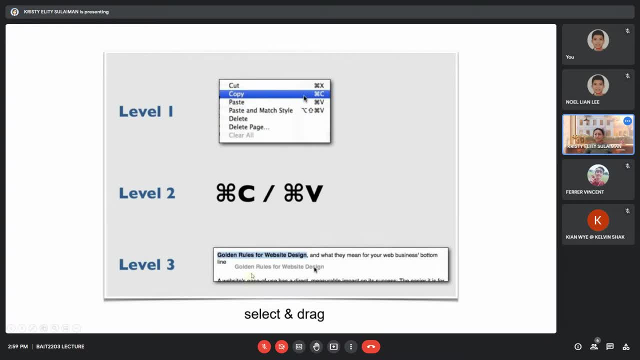 other other apps? okay, uh, do you all have any um experience using mac os? anyone using mac os? okay, okay, so, okay. so, if no, yeah, if you have not seen how macbook works, if you like, have transition, let's say you get, you got a present on macbook. 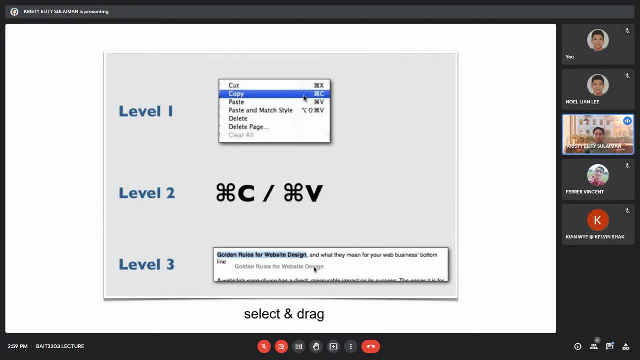 example. so, uh, you have been using, you have been using windows for your life. then you don't have any experience using macbook. okay, so maybe you will have, because the systems are different. so the view of the view of the apps you have also have different, functionality, different, uh, different. 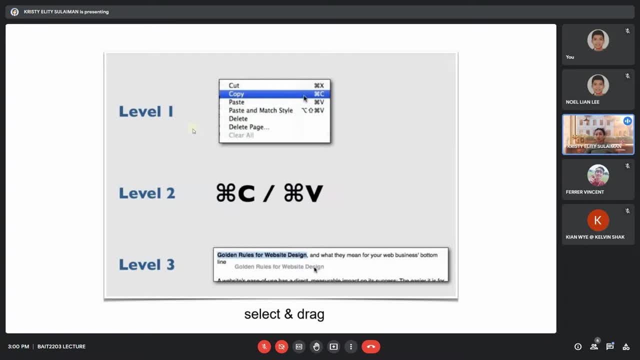 different if we give you different direction, right? so, um, for, because you all has always been using windows, so you might, when you use, uh, when you like, transition, transition, transition to use macbook or macos, you will find that you will use as topic of questions, will like, you will use the shortcuts that we use in windows, in mac, in mac os, whereby it will not function okay. so that's why, uh, my point here is that your past experience also same for YouTube. you can also useилоes, which you 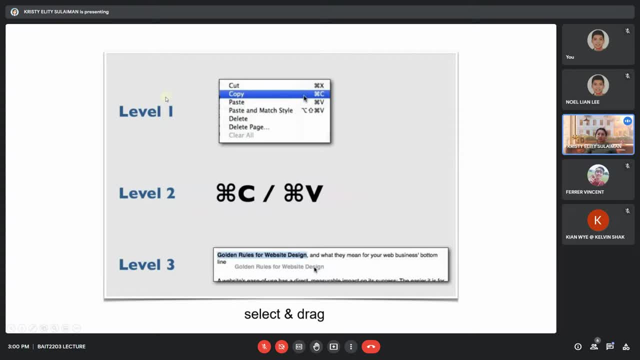 is important when you want to design your system, okay. so that's why, for when you design your, your system, for your project, you need to know your user, what, why are you? why you indicate what is the machine or what is the smartphone that you use, the use, okay. so let's say, if you want to design, 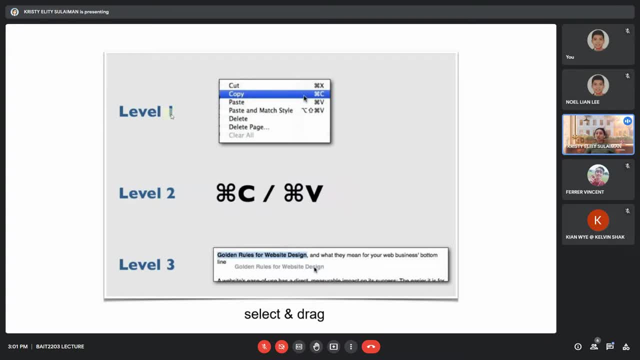 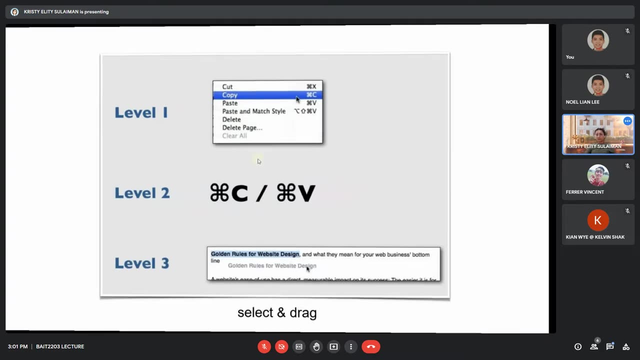 for, uh, apple user, for example. so you need to look at how apple present their design and then you switch your design to their, to that, to the, to mac os design, right? so similar goes to the shortcuts. and then we have this one, um, this one. i will not explain this. 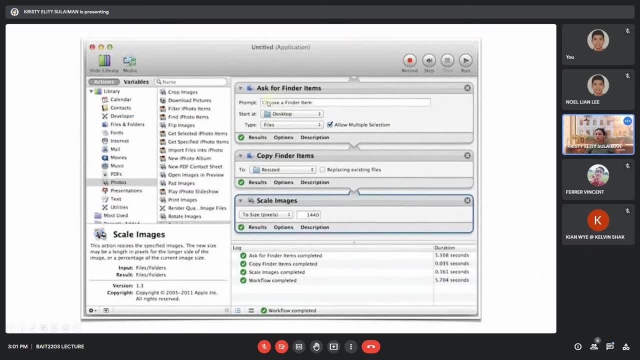 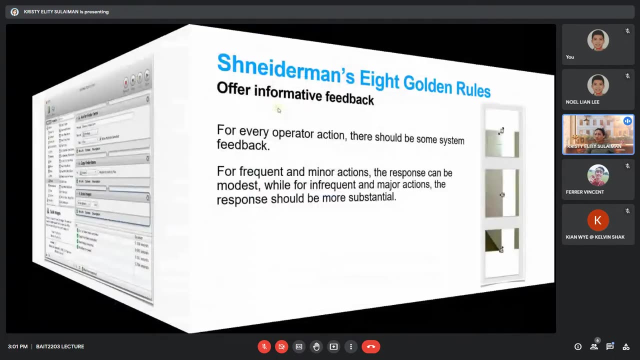 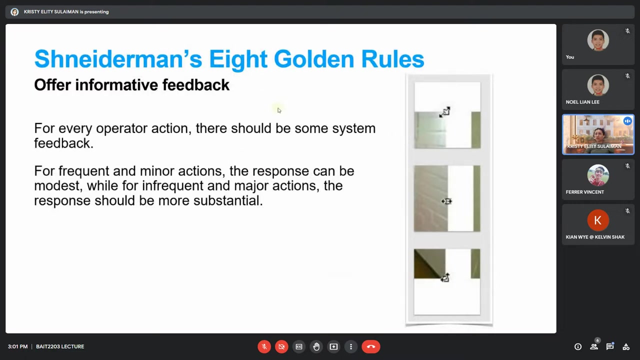 this one actually an example. this one is from mac os, basically, uh, some, uh, this is the functionality that you can also find in mac os partition. i believe is the previous mac os version. okay, so the sec, the, the next golden rules of a certain snake demand we you need to offer. 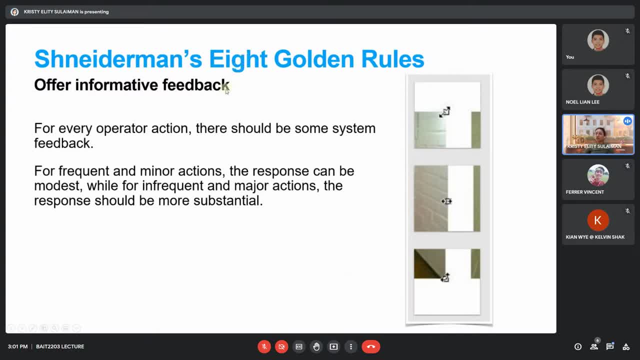 informative feedback. okay, so for every operation like you have some, like the usual, where you finish, uh, keying in all the details, or maybe for booking and already in for like the access activities, right? so you need to provide feedback. so that know that. oh, I already done the thing right. so for frequent and minor actions, 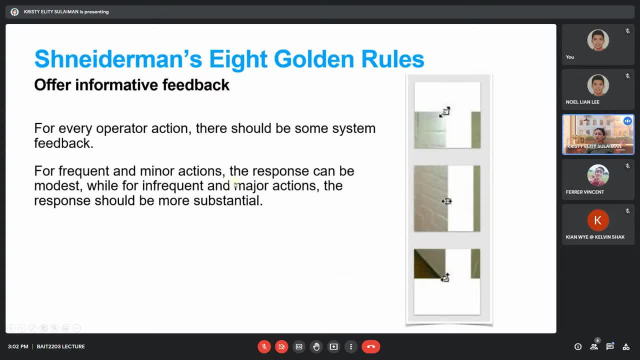 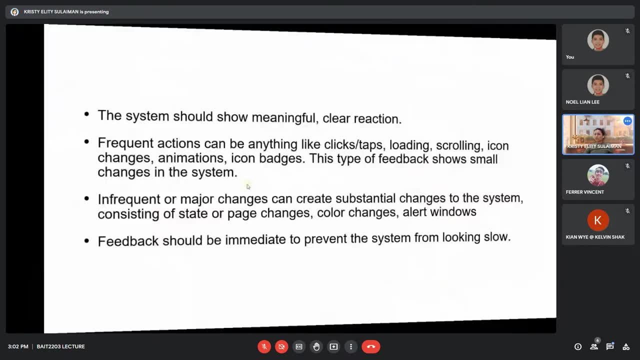 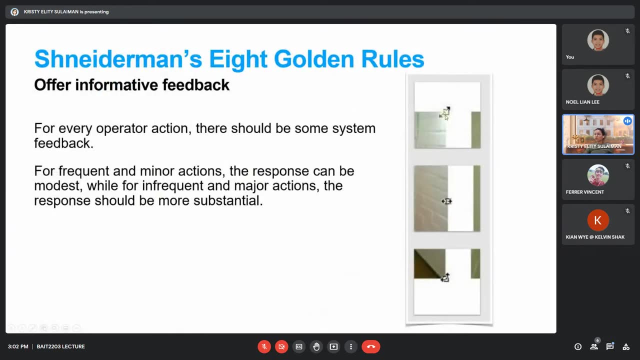 the response can be modest or while for infrequent and major actions the response should be more substantial. okay, so like this one, right. the example here, the cursor here, shows you that if you use this edge of the picture, you it will drag and make your picture bigger. if you put at the side, it will. 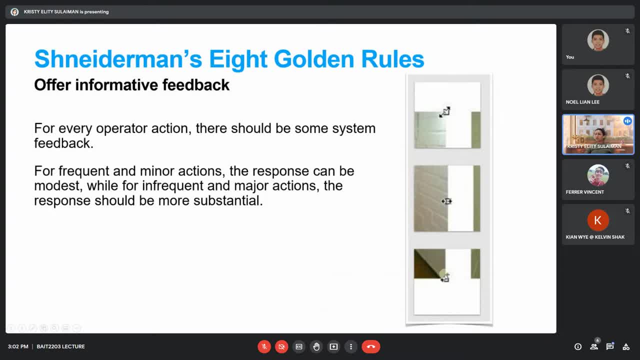 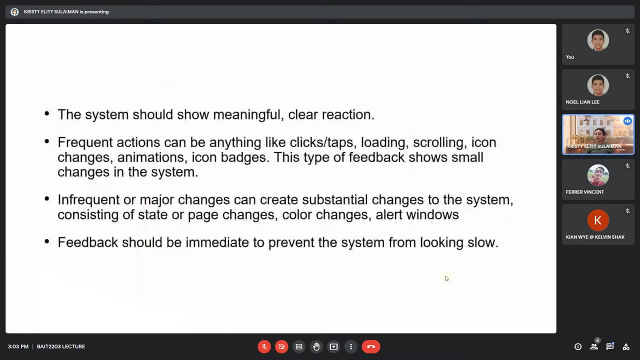 stretch your figure and similar cross to this one. okay, so this shows that you give feedback to the user and telling them what they can do with this function. right, so system should have a meaningful and clear reaction. so frequent action like click, loading, scrolling icon, changes animations, so this type of feedback it. 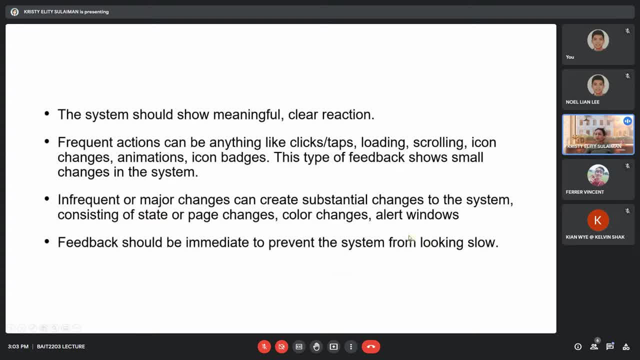 shows small changes in the system and then a type of major changes you can use, like a page changes, color changes or a lit window. so feedback it should be immediate to prevent the system from looking slow, like, for example, when you click on submit button. okay, after submit, you should directly get the feedback. 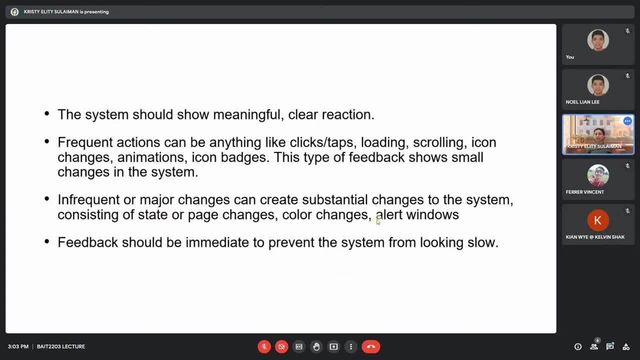 that the response of submitted something in there right. so you need to design a feedback whereby you inform the user what have been that the system already get what you input into the system and make sure that feedback is immediate to prevent that showing they prevent your system for. 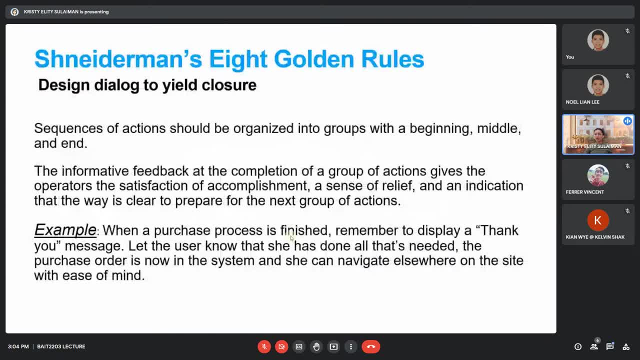 República. Wait a minute. rules is that you design dialogue to give closure, okay. so let's say example: when you do um e-commerce in e-commerce, like uh, buying things on website, uh, or maybe like um order, like you want to schedule for a movie tickets, for example, you want to buy movie tickets, so they there will. 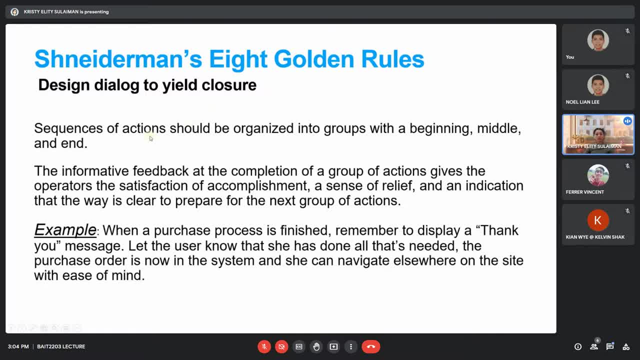 be a sequence of actions, right, like you log in and then you select your movie, select the day, select the time and select your payment, right. so that are the sequences of action. so those actions should be organized into groups with a beginning, middle and end. so informative feedback should be uh given, uh at the completion of a group and 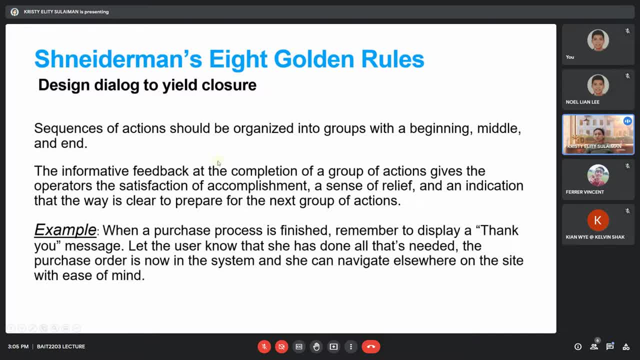 it will give the users a satisfaction of accomplishment, so also a sense of relief, and it gives indication that you can go to the next action right, for example, here, when you do a purchase. also, when you purchase, uh, when a purchase process is finished, you need to give a display, a thank you message, so that, uh, that means that you give feedback to the user. that 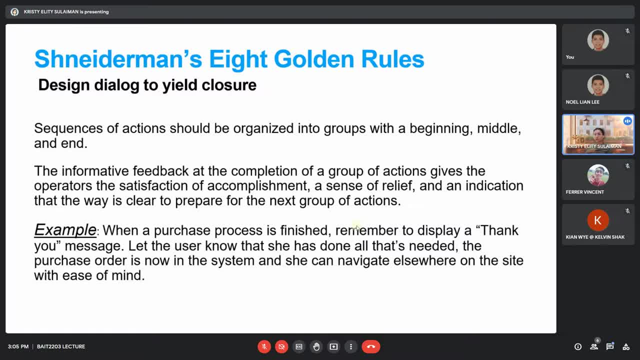 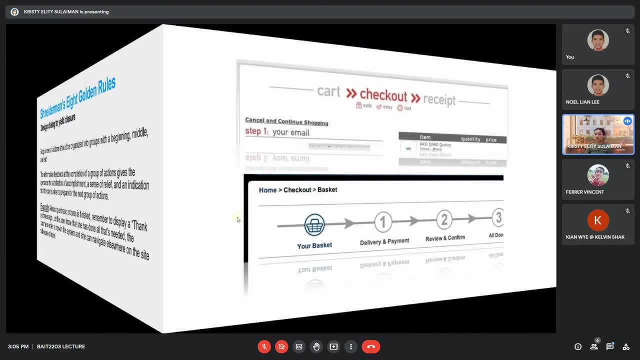 okay, we have received your order. we proceed now. thank you, right? so you want to let the user know that the user has done all that's needed, right? so this is an example of, um, how you can use these rules in you designing your system. so here you. 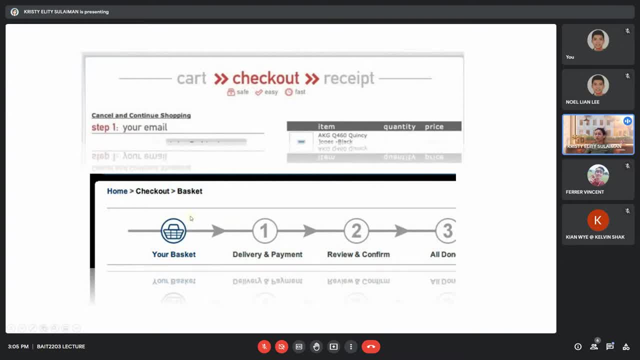 have this action. so you must, you have. you have your card, the basket, your basket card, and then you pick your delivery, delivery and payment, and then you review and confirm and then all done right, and then, uh, this shows your um, grouping of grouping of action. okay, so similar goes to this one. 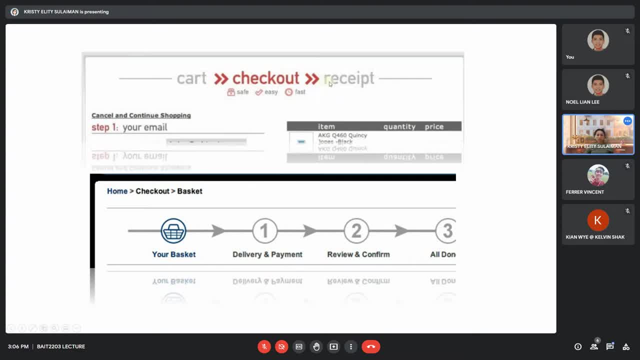 if the card you have to check out and you provide a receipt. okay, so if you have, if you have used banda or credit, grab food or grab delivery or great car. uh, you, you also can notice this that, like, if you buy food, you pick, you want to buy a closer, or you want, you want to. 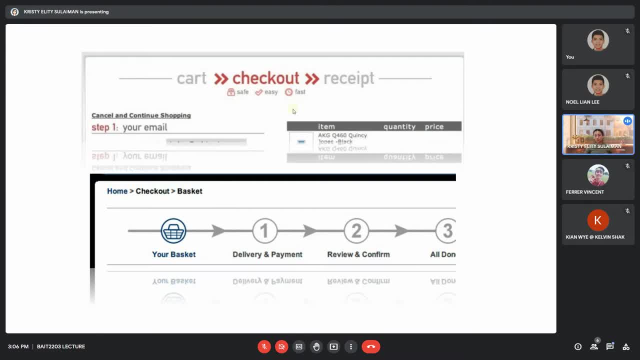 browse trademark. or you want to browse great food, right? if you want to buy food, you go to grab food and then pick your restaurant, you pick your food and then your payment and then up until you click on order, okay, so if you have experience on using those, those food delivery system, next time, if you 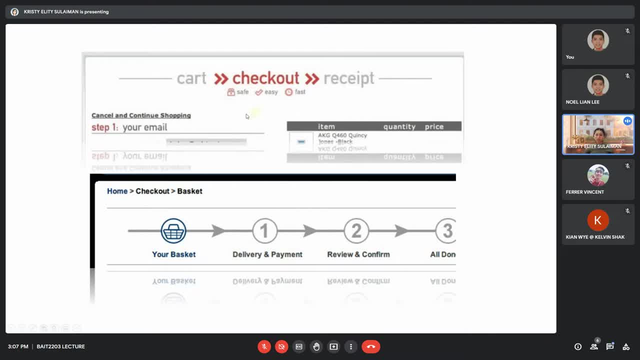 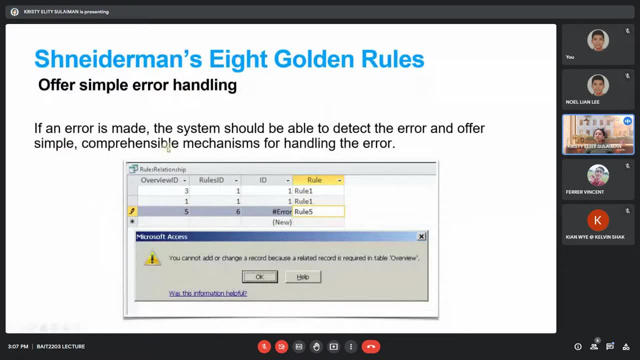 access it again, you try to see the actions that is done in that system. and then the next rule is offer simple error handling. so if an error is made- so you see the system- it should be able to detect the error and offer simple, control, comprehensible mechanism for handling the error. yeah right, so this one, this one. 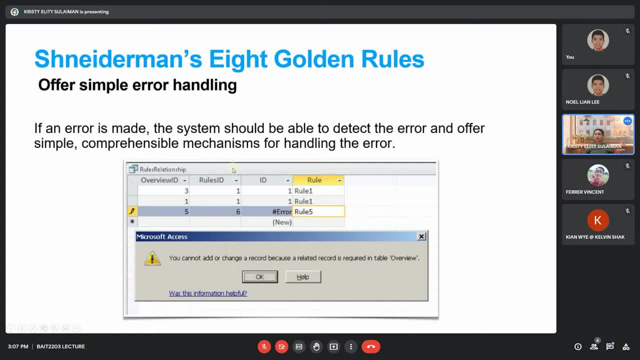 is an example of. I think this one is microsoft, microsoft project. what we here, microsoft, create this database. you know, you Cosmos access. okay, so this is the view of Microsoft access. yeah, so, Microsoft, this is Microsoft access. so let's say, you design a siblings relationship between is of the indus ID, so you are given on to not comebroken. 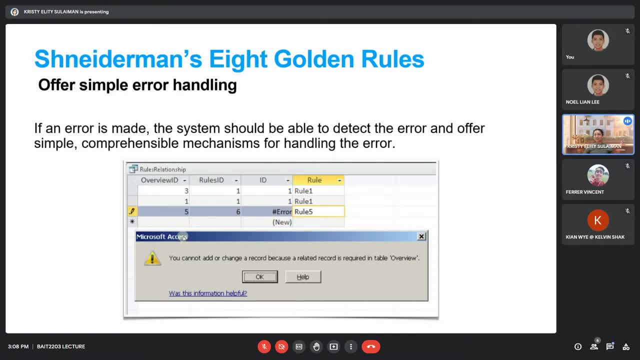 it's the future. So Microsoft Access gives you the error, like if they found that there is an error in your relationship. you will be given an error handling message. So you cannot add or change a record because a related record is required in Table Overview. 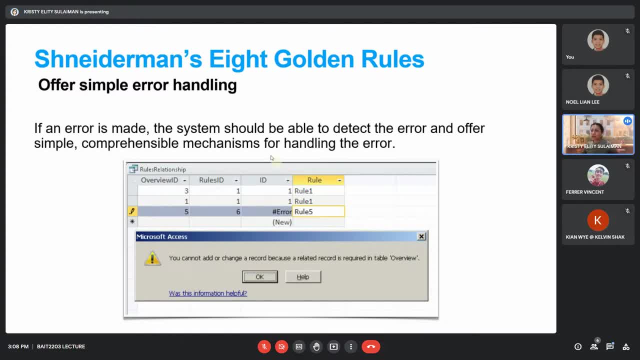 So this one is very simple and you can understand why this error happened. So it's actually also tips for you. when you want to create your design for your assignment or for your project, You can use this type of error handling. You can show it in your prototype later on. 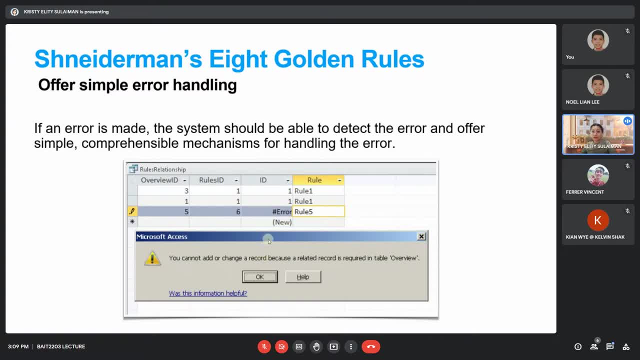 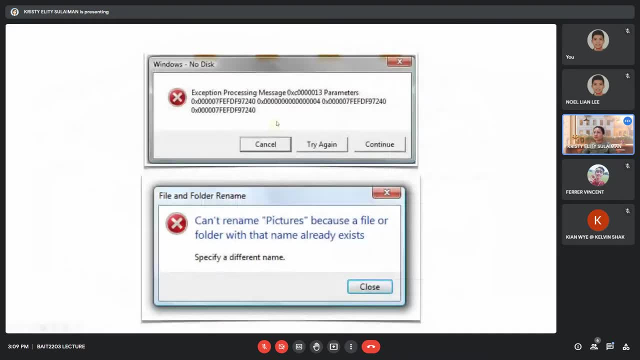 So here it's very comprehensive and it tells you why the error happened. So another example here would be something like this and something like this: So Windows Node, So this one is not human-readable, right? So you don't know what is the exact. 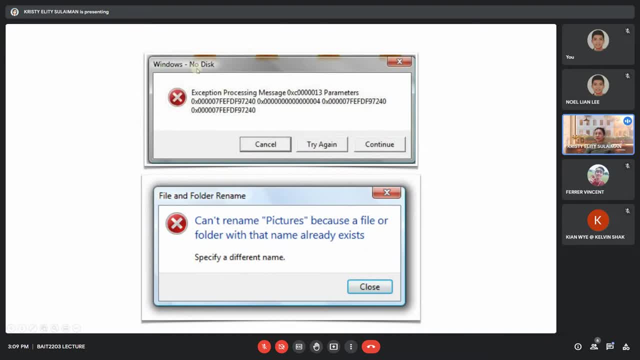 how do you detect the error? It already mentioned here, Node Disk. but the explanation here, like it's, only the computer will understand this right, And then you can cancel, you can try again or you can go to. It's up to you what button you want to include in your design. 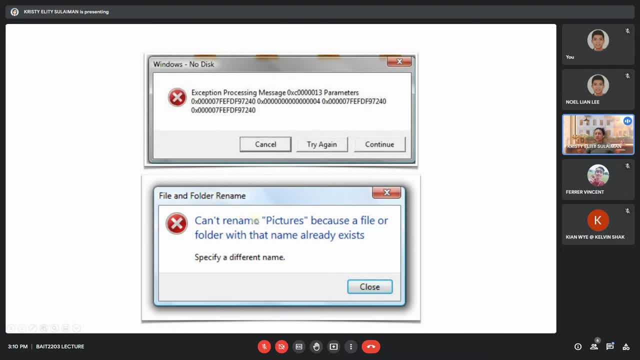 And also file and folder name, so you cannot rename because the file or folder with that name already exists. So it gives you solution. So this pop-up will give you a solution. You need to specify a different name, right, so that you know what to do next. 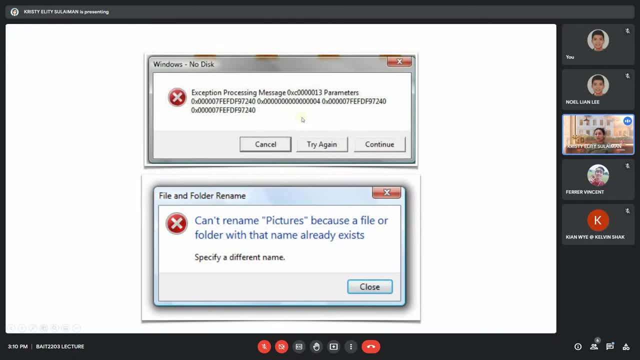 But this one. it doesn't tell you what to do next. OK, So you decide on your design, how you want to give, how you want to help the user to do this. So you need to understand what is the error that they face. 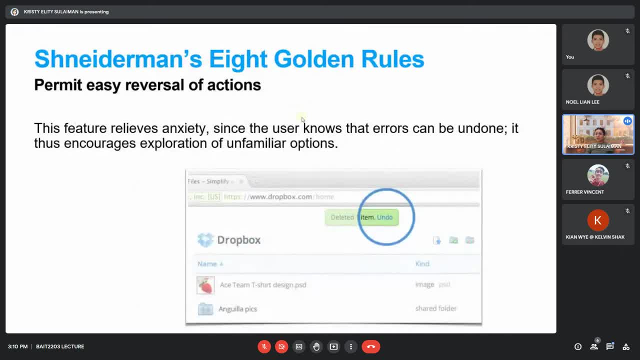 So the next rule is to permit easy reversal of action. So this one is something like undo. So this feature, it relieves anxiety, Like maybe you accidentally deleted an item. You can provide reversal of action, which you can provide a button or an option. 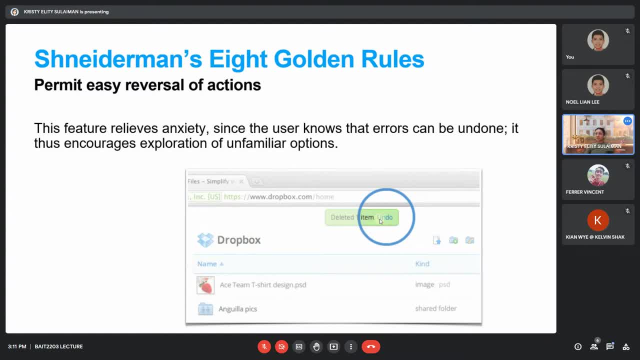 to undo the action So that the user don't feel anxiety that they have accidentally deleted the item. So previously this reversal of action is not always included in the system, But nowadays I can see improvement in our system, especially for Gmail. 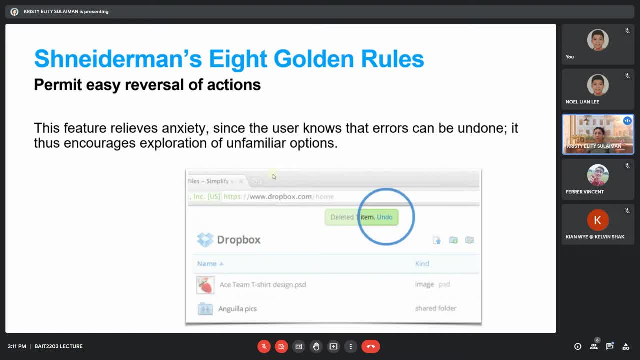 Gmail. if you accidentally sent out an email, you can still undo it in 5 seconds or 15 seconds, OK. So this reversal of action also helps users to be confident when they use your system. If they make any mistake, they know they will. 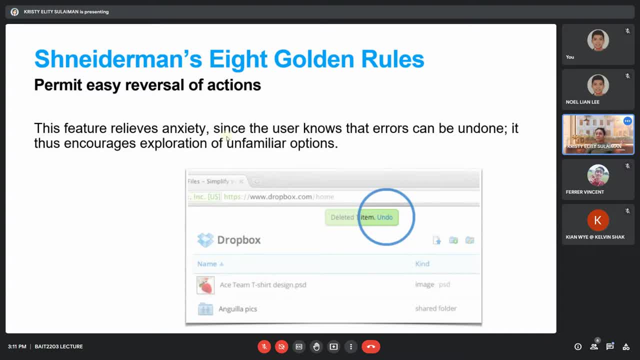 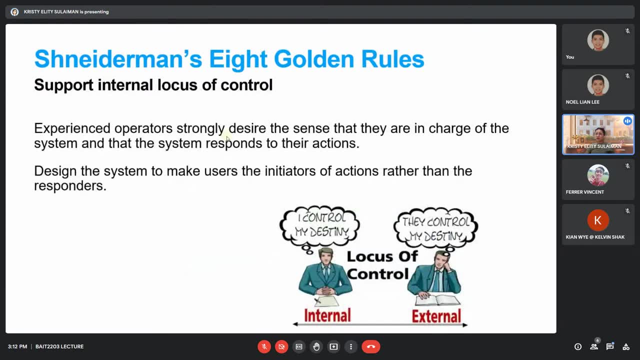 be able to undo the mistake. OK. And then the next rule is that to support internal lockers or control, so experienced operators or experienced users, they strongly desire the sense that they are in charge of the system. OK, So internal lockers of control is. 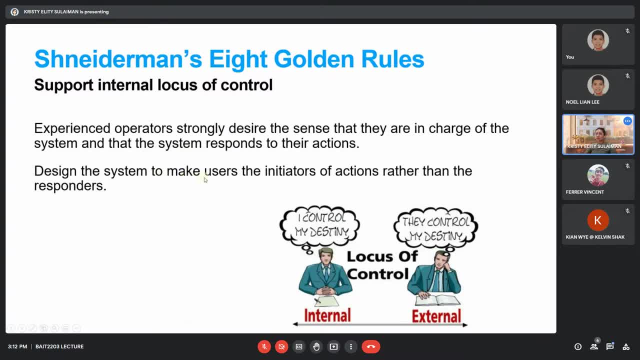 whereby you want to design the system to make sure users the initiators of action rather than the responder. So you want to make the user initiate the action rather than the responder. OK, So it means you use your internal lockers of control when you want to use the system. 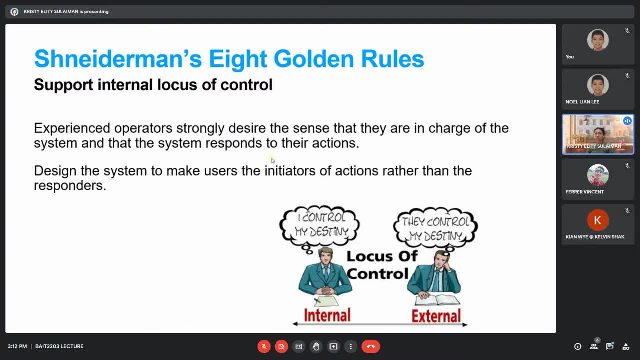 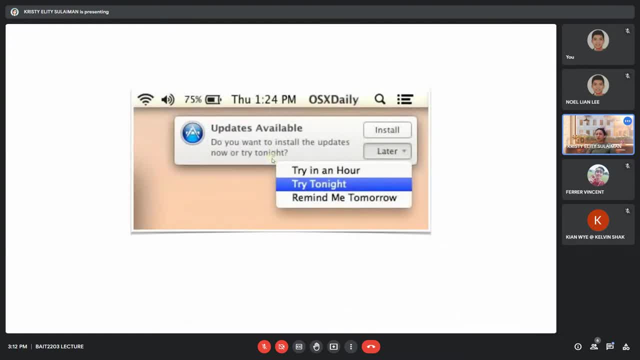 So here you need to take this into consideration when you want to design your system, For example, like this one. OK, So this one is a view from Mac OS, But this one is also available in Windows, or Let's Happen. 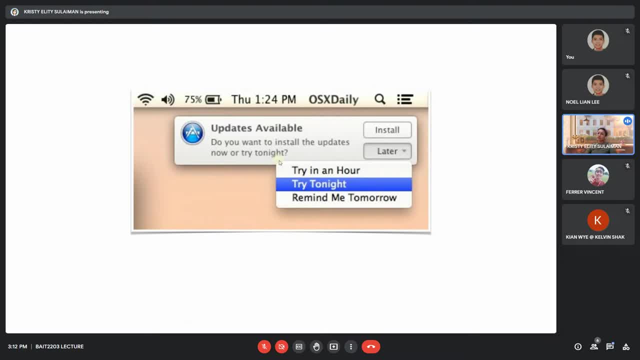 If you enable the notification to enable the notification of system update, you will see this right. So you give You give the user like flexibility on how to do the how to install the update right, So you can previously for Windows. 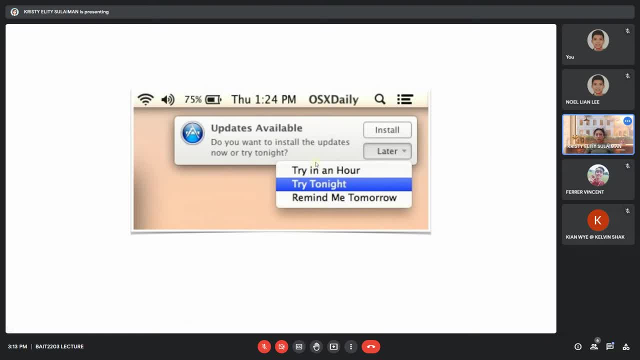 you don't have this option, Like I, want to update now. The update must run now. Don't shut down your PC, Don't shut down your machine. OK, Those are. that was previously OK, But Microsoft already improved. 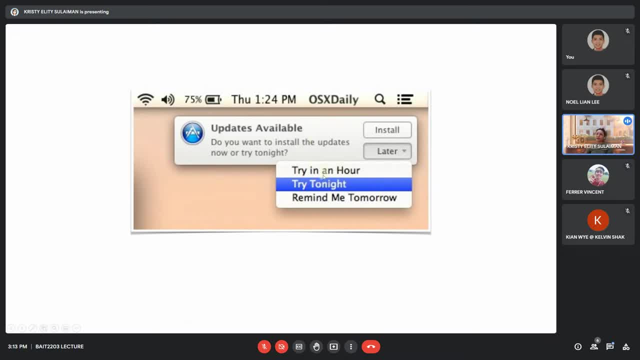 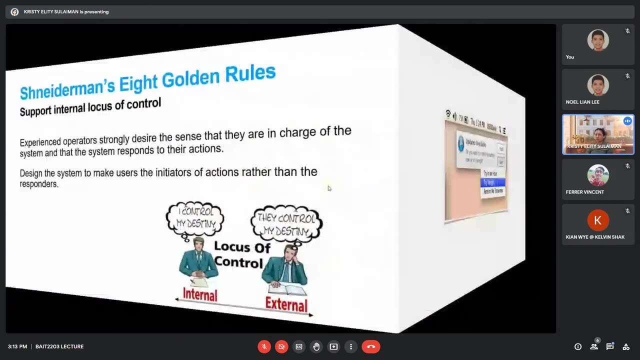 They give some kind of Choices. OK, So you can try in an hour, you can try tonight or you can remind me tomorrow. OK, So this one is an example of internal lockers of control. So you have the control towards your system. 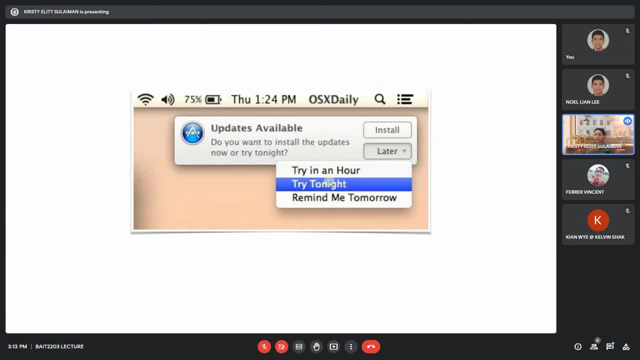 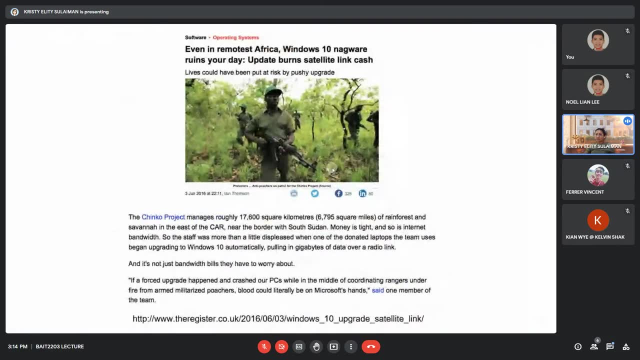 So you can allow this to user so that they are comfortable using your system. OK, OK For this one. this is just an example of article We buy in Africa. when was this 2016,? Windows, Windows, like Windows, like they donated. 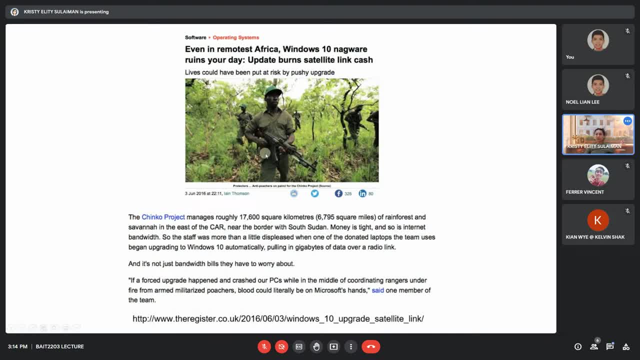 a laptop for to be used by these rangers in in in the jungle. They use a satellite satellite link to get internet And then, at the time we buy, they run like they run a, which are missing a machine. 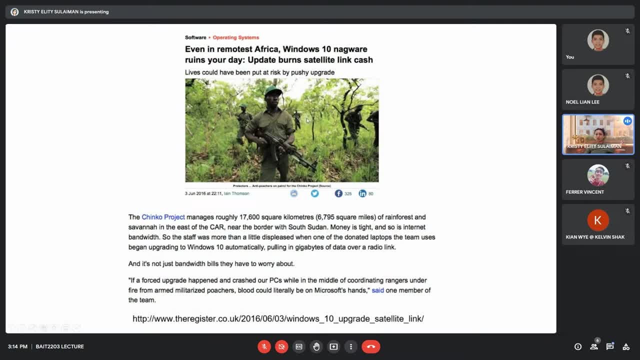 whereby they, the rangers, go into the, into the, into the forest, and they, but when they want to detect, like, detect the movement of the illegal hunting in the forest, all the, all the machines that they, they, they got from the, from the, from those donated. 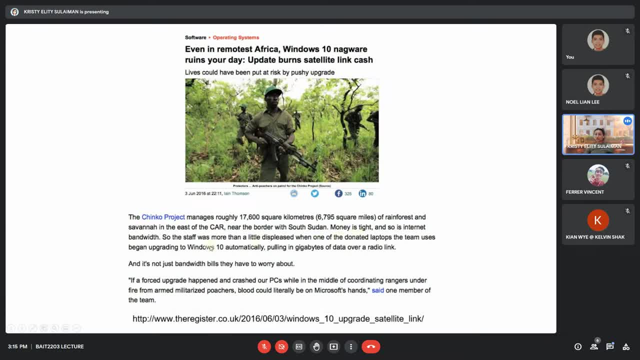 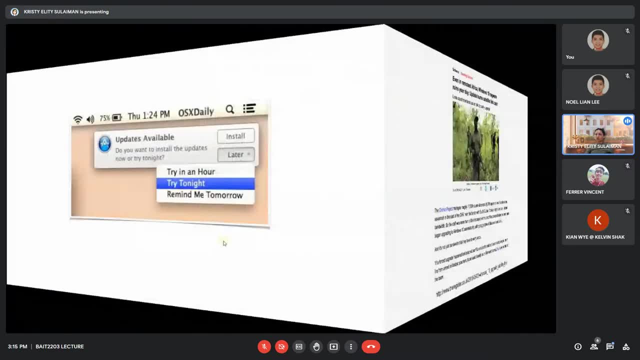 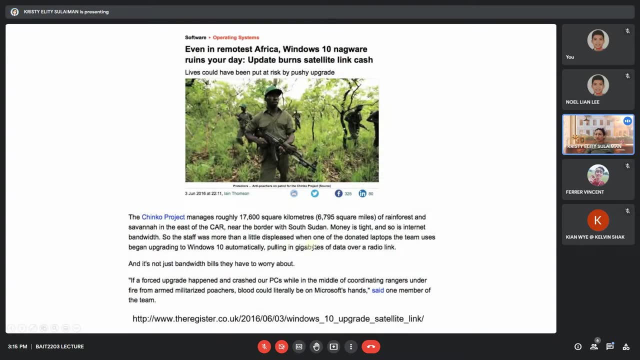 laptops, So People, you can get m aussi. So now you have to create like a layer with a satellite. So, ah, okay, Okay, Can, can, can be vended, as you can see They and there they, they. you know, after they've, after they grinding, uh, it goes there. 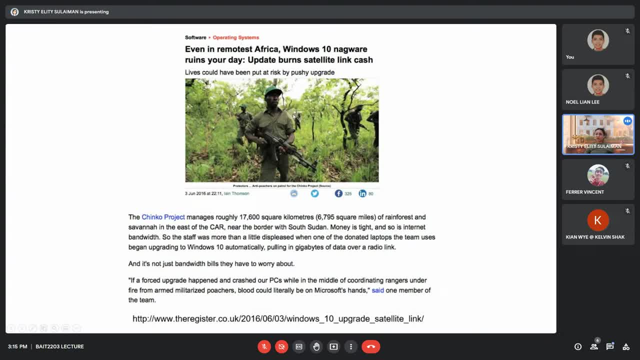 Yeah, There is what I. ii mean Yeah, Yeah, when we were used, okay. so this is just an example of a real world where windows 10 has the windows update has affected these people. i guess we can refer to the full, full article from this link. 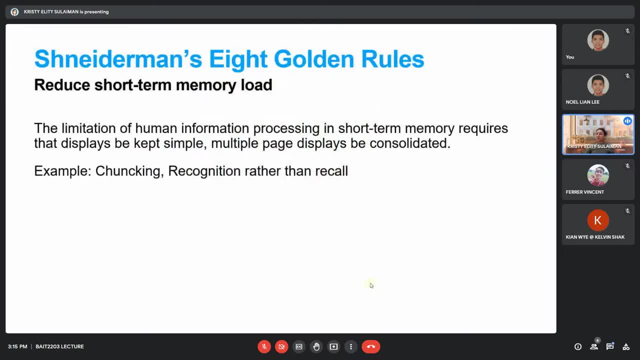 and the next: uh, so this is the last rule, so this one: reduce the memory load. we have discussed this previously, so you need to make sure that your design, your ui design, reduce short-term memory loads, which, um you will, you can use chunking without see behind. 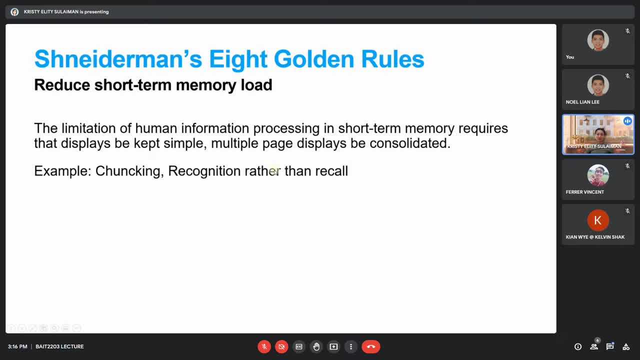 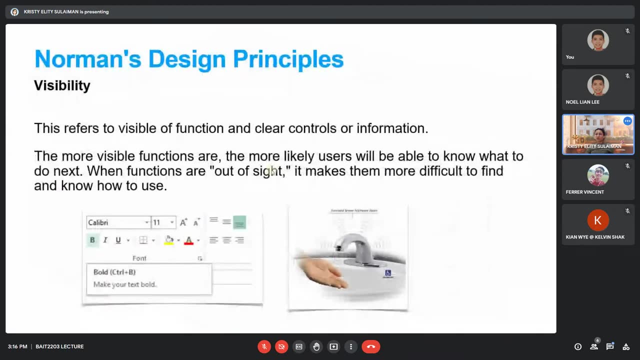 tanking. and then you use recognition rather than recall. okay, so this one we have discussed uh in the previous lecture. so, other than this schneiderman at golden rules for ui design, we also have the normans design principles. okay, so we have several uh design principles for. 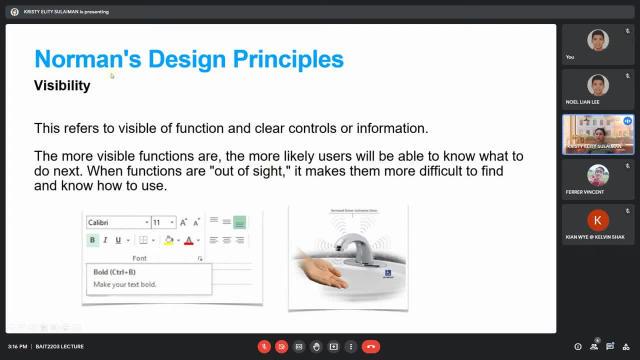 and these, uh, normans and another expert. so this one schneiderman is also another expert of hci. so now we look at norman's design principles, so some of the principles that you will see next. it might be similar to the previous one, okay, because different, different. 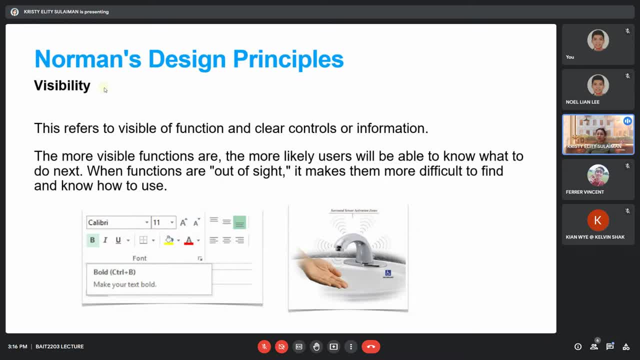 researchers, right, so they can have, they can have, uh, similar ideas on how hci should be, how hci should implement ui design. okay, so we go to the first one: visibility. so this visibility principle refers to the visible visibility of function and clear controls of information. okay, so like say, for example, like you want to use the volt function on, 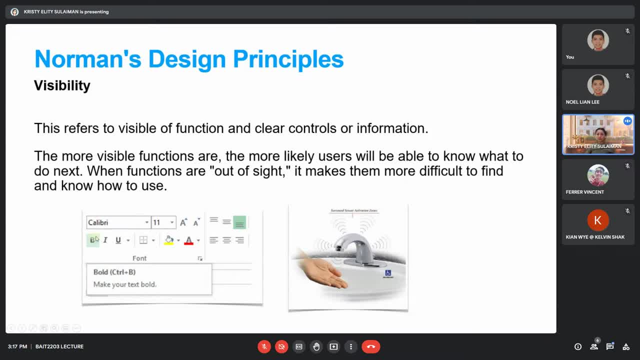 Microsoft Word or Microsoft PowerPoint or maybe Microsoft Excel, so you can directly hover your, you can directly go to the menu and just click on it. so let's say, if this V function or default function is like somewhere under the file menu, right so you will not be able to like, you don't even know that you can. 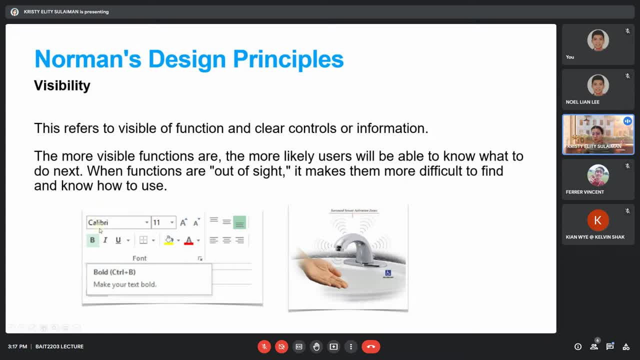 hold your text, let's say, if you are a new user. okay. so another example here is: this is a sensor that water. I think you will also have experience this, like in hotels. some malls also use this sensor activation tap water. so like you don't know where to put. 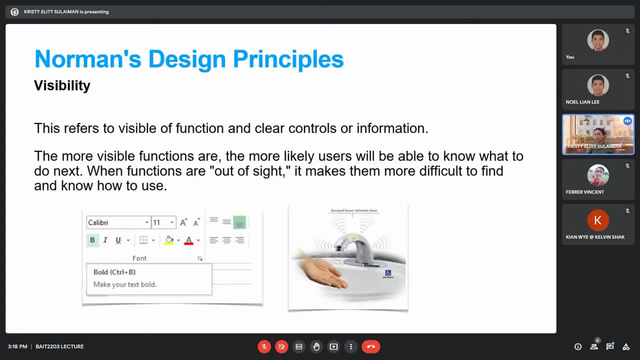 tap water. so like you don't know where to put your hand, like whenever you keep looking for the activation zone. so because the lack, the design does not show you where you should put your hand right. so some some um five might show you where is it where you should put your hand exactly. some might not okay, so when it's out of sight, it. 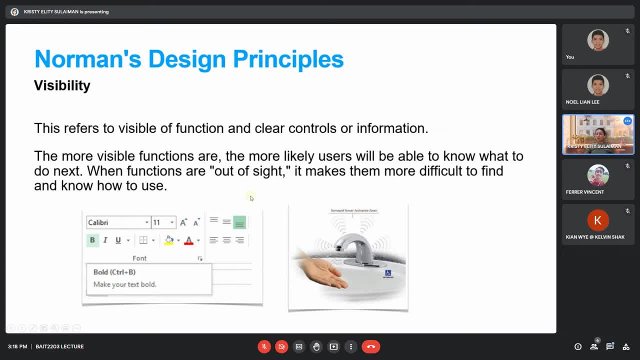 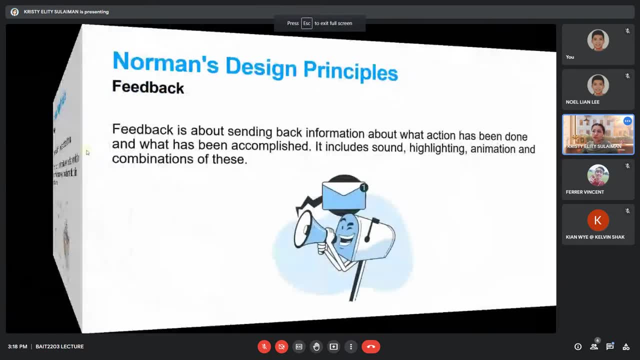 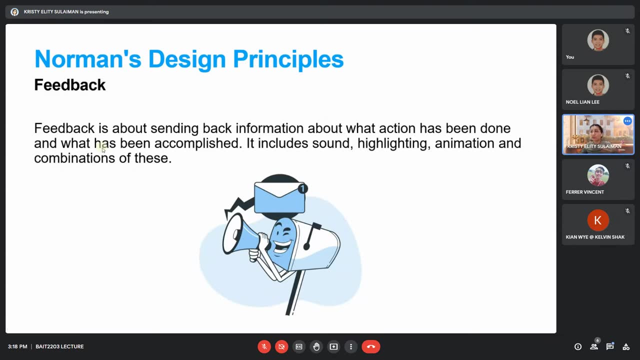 makes it. it makes you uh difficult to find the feature and you will not know how to use it. and then the next one is feedback. so this one is similar thing with as nine dimensions now. so feedback is when you want to give, give information to the user: what action has been done and what has 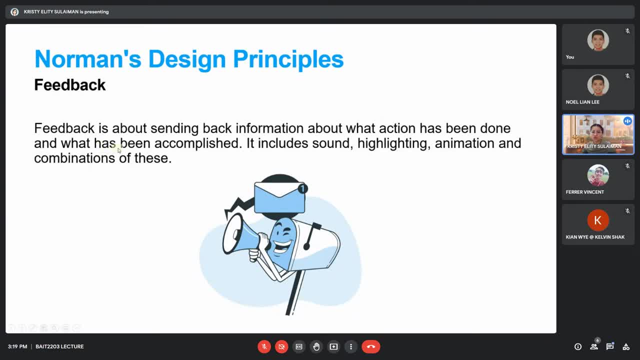 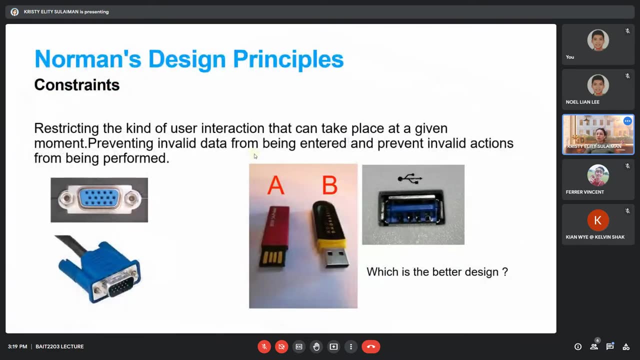 been accomplished, um, after the user do something on the system. it can include sound you can use, you can use animation or a combination of this or maybe others. okay, and then the next principle is constraints. also constraint is when you restrict the kind of user interaction that can affect us. 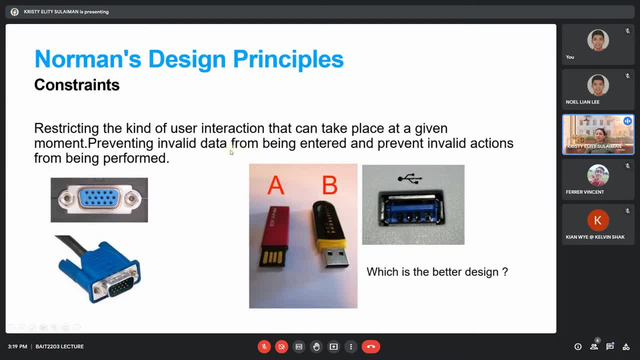 at given moment. so you want to prevent invalid data from being entered and prevent invalid action from being performed. okay, so you have, uh, you, you look at constraints um whereby you decide on your ui design, on your ui design. you can also use this constraint, for example like: 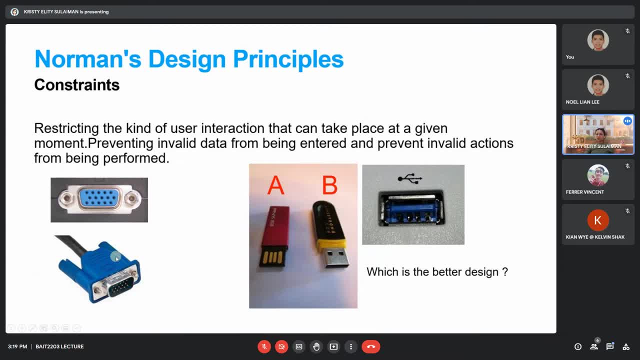 this one, right, so you need uh this way. this one is obj cable. um, you need to like follow the pins for you to be able to plug it in. similar goes to this one. so, uh, there are two types of this are usb, so you can use uh, either this or this. so this one i sometimes it's very hard to like to. 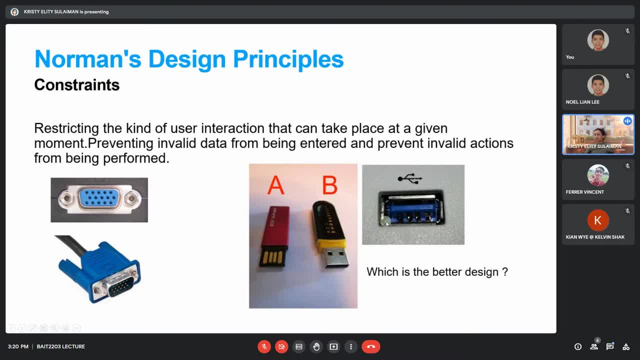 find the head right. you don't know which which side like which side to put in, okay. so most of the time you will like you will put it in wrongly right. so these are types of constraints like uh for your ui design you can set like uh. maybe like uh for user that already make. 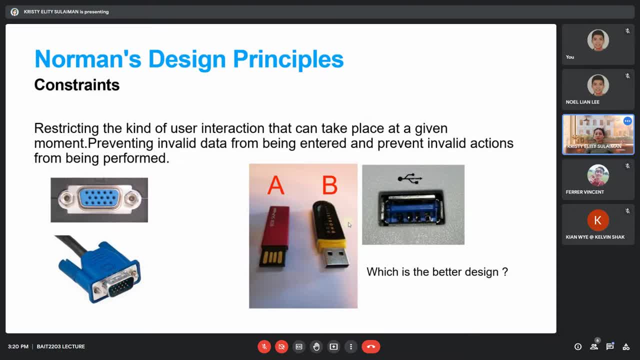 uh an order they they cannot like. they already make payment. you cannot go back. example: so what you can do on your ui design is that you put the constraint on the payment button. you, after it's clicked. once you put a constraint whereby it will be grayed out means it cannot be. 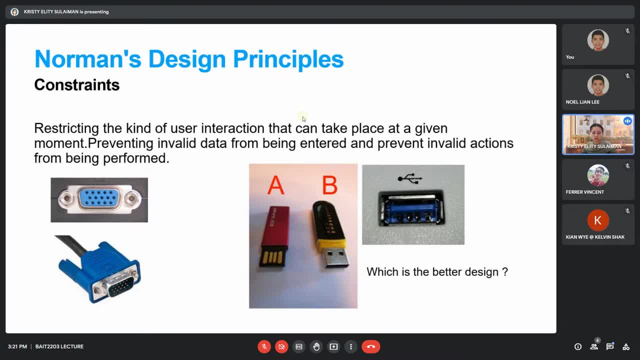 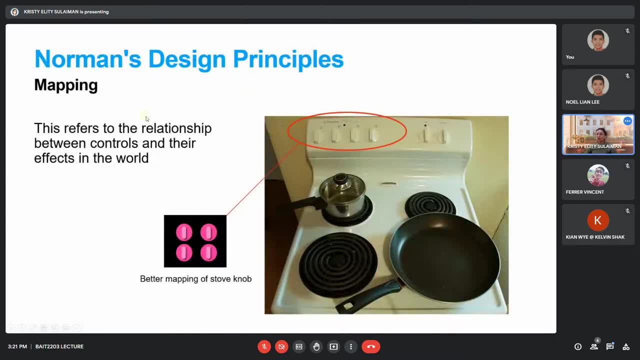 clicked anymore. okay, so that's an example of constraint in ui, and then another one is mapping, under this norman's design principle is mapping. so this one. it refers to the relationship between controls and their effects in the world. so this one example, like these notes, uh, are for this four. 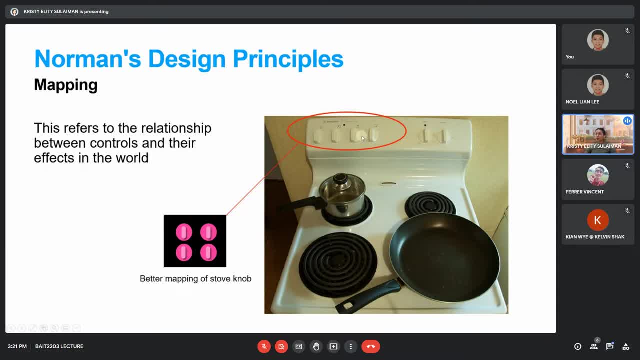 stuff. okay. so if you design it like this, right, you don't know which is which. okay, so, better, mapping of the stock knob should be like this: okay, so the this way, you will know, the user will know: uh, this one is for this, this one is for the bottom line, this one is for this and this one is for this. right, so mapping is helpful. 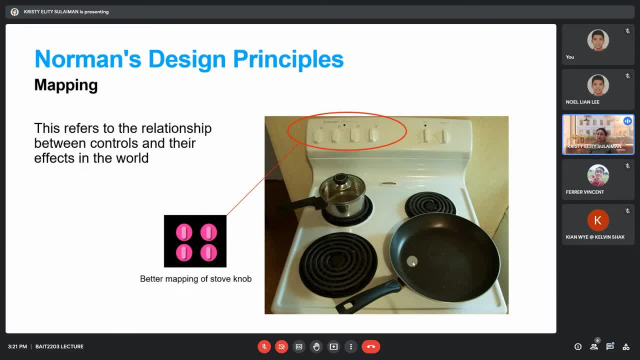 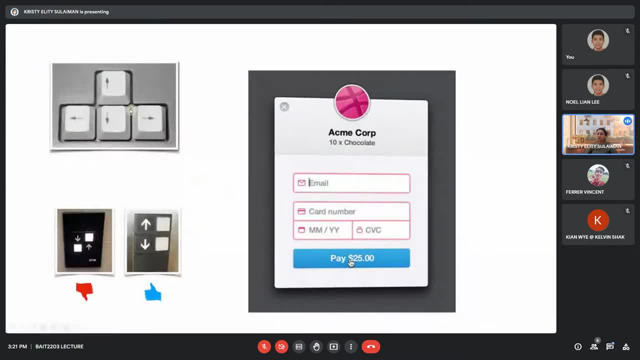 so it is basically helping you to underst, to help the user um use your past experience to your system better. okay, so example of that is this one um. so like what this is? we go to this animation, so this um, when you pay 35 dollar, right, but it gives you like shaking, shaking animation. 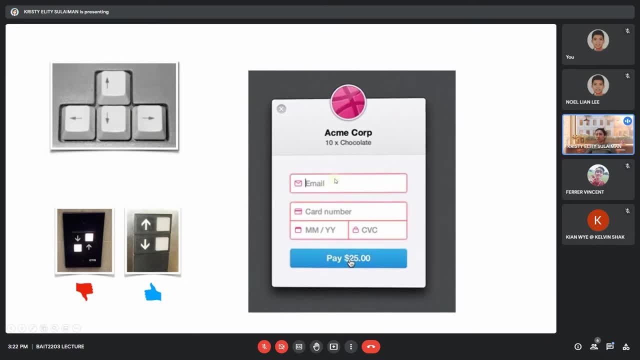 okay. so in our experience, we know that if it's shaking and it's right, something is wrong. right, so that's how you, um, that's how, uh, you can apply. mapping in your ui design means to give like feedback to the user. um, according to their past experience, like, if, like. 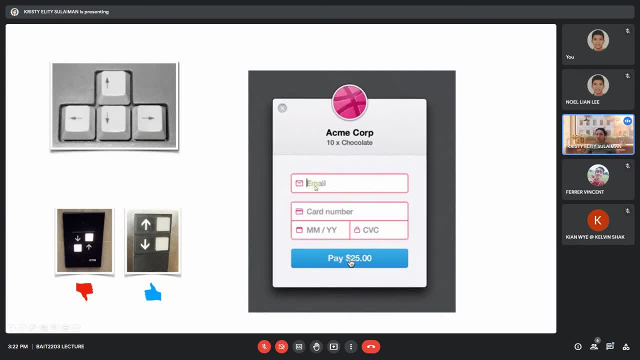 it's shaking means like it's no, cannot proceed, and it's. moreover, it's red and it's blinking, right. and then for this part here. so this one is referring to your experience. so, when you use your keyboard, you always uh, press up and down, uh, like this. okay, so you will prefer to have this. 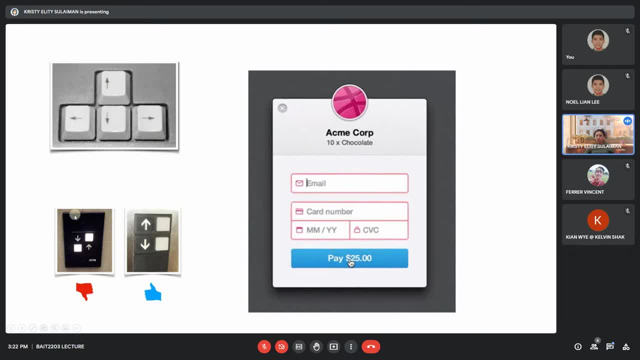 design rather than this design. okay, because this design it's it's not familiar to you. you might press wrong button, right. so this one is like, it's more accessible, it's more understandable because you have been using it on your keyboard, okay. similar thing when you do gaming right um your keyboard. like, let's say, today you play at your home and next. 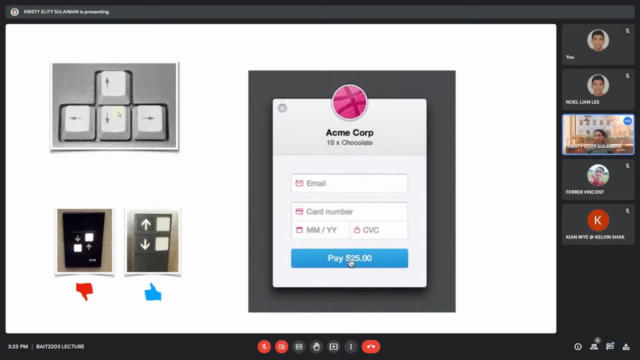 day you go to play uh at the cyber camp or at your friend's home, you will use your friend's keyboard, but your keyboard keyboard and the key on your keyboard is uh. placement of your key on your keyboard is not the same with what you have at home and with what you have at your. 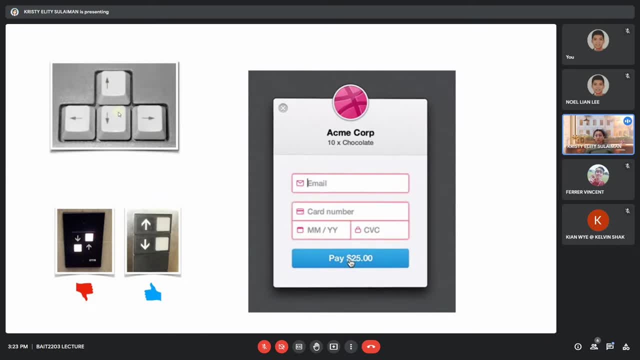 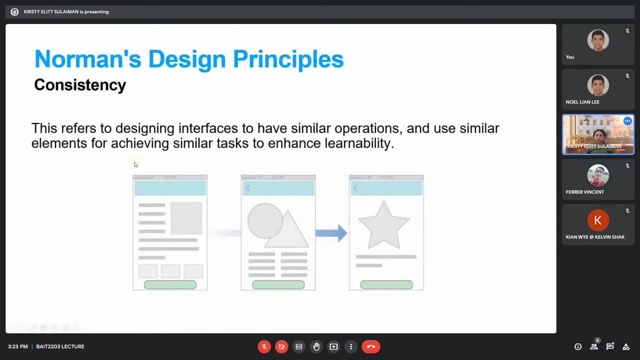 friend's home, so you will have difficulties on controlling your games due to the uh key keyboard differences. okay, so that's it. that is an example of a fast experience, and then another one is consistency. so this one is really similar with the the previous uh principles, so it refers to designing the ui to have similar operations. you use similar. 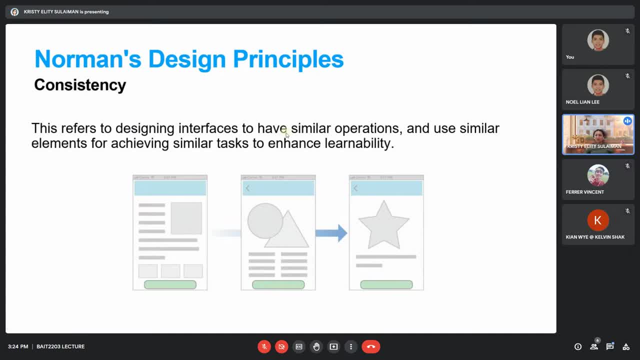 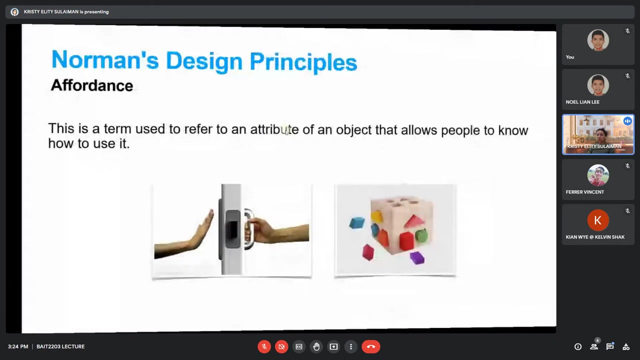 elements to achieve similar tasks, to enhance the ability. okay, so, for each like, for your term, like every page should have the same font color, you should have the same button size, right? so, uh, you can apply this consistency to help your user enhance their. and then affordance. so what is this affordance? so this is a term that's used to refer to an 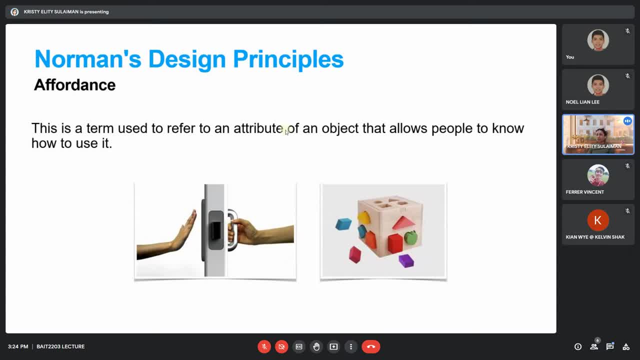 attribute of an object that allows people to know how to use it, for example, like this door. when you give like this: uh, if it's like this you, you need to push it. if you have this handle, you need to pull it right. and then this one also are you. you type the blocks and you put it in where. 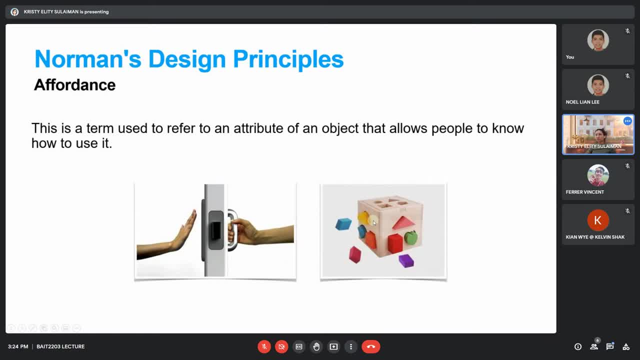 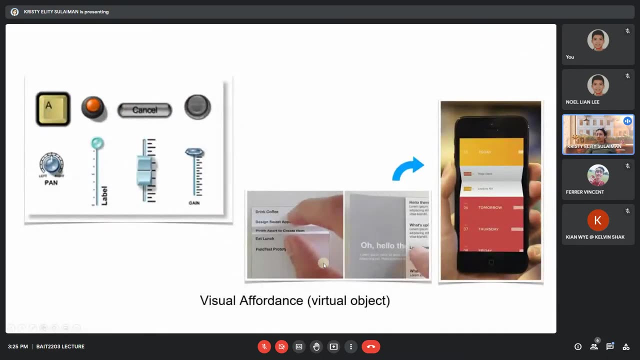 it belongs, right. so this is affordance: you, you give or you provide a ui that will allow people to know how to use it. so an example of that is this: okay, visual affordance. um, so here you have a paper right, the characteristic of paper. you can. 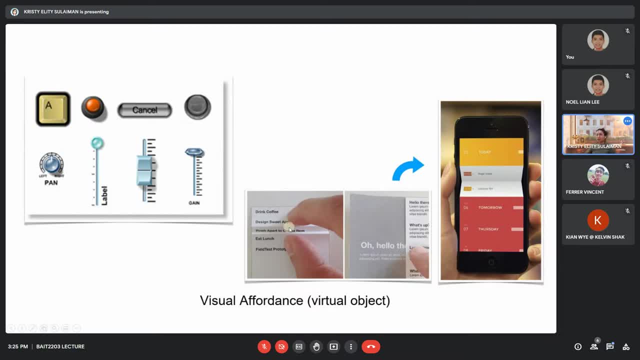 fold. you can fold a paper like this and you can apply this also to your smartphone, to your app. okay, so this is something like: uh, this is for from the real world experience converted to an app. okay, so, this is like um, a paper fold. okay, so you can apply this kind of. 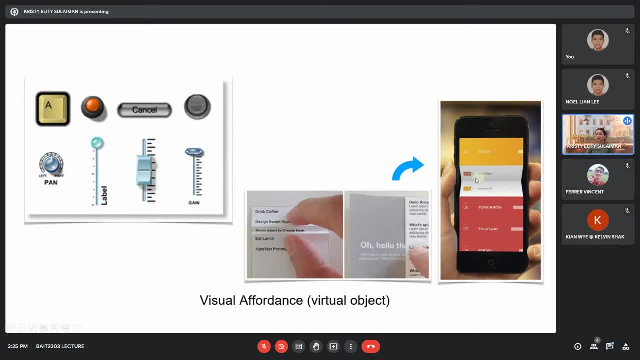 things in your ui design also like this: um, you can include, like um, more information on your design. like, uh, the pen. and then this is the, like the four letter, a, keep on the, a cancel. and then this is one is to like to lower the volume, um, lower or make it maximize the volume. and also okay, okay. 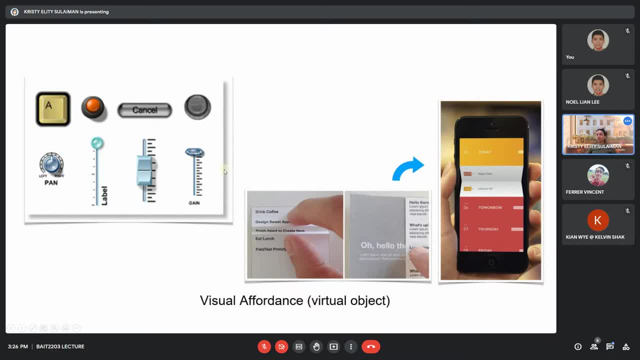 just uh, basically, um, for you, for you to have an idea on how you use experiences in the real life. you convert it into the system so that the user, they, they feel more comfortable when they are using the system. so those are the ui design guidelines, according to sniderman and also. 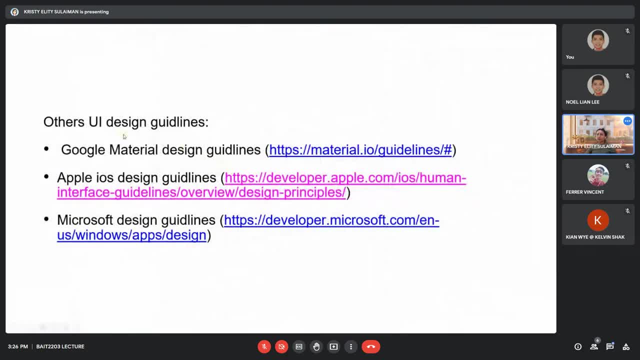 norman, so you can also refer to this uh ui design guideline. so i i believe you will get more information on how you should design your ui from this website. you have google natural design guidelines. you can refer to this, you can google this, and then you have the ios developer and also. 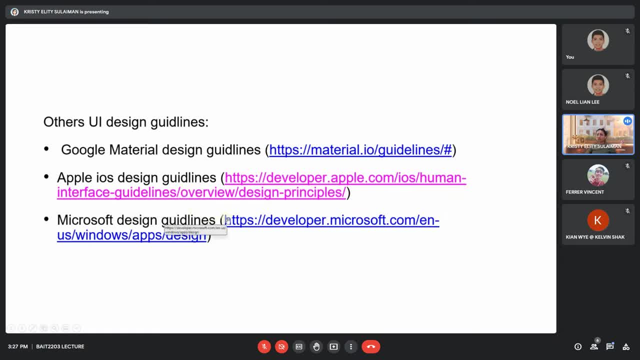 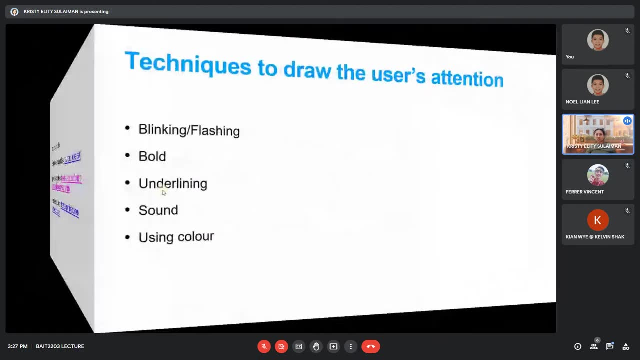 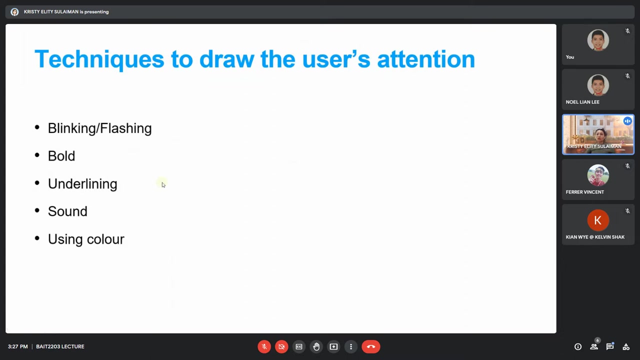 also design guidelines, right, so you can refer to this um to have more understanding on how to do this. okay, so another part of this lecture is, uh, we will be discussing on the techniques, on how to draw users attention when they are using your system. so you can use this: blinking or flashing. 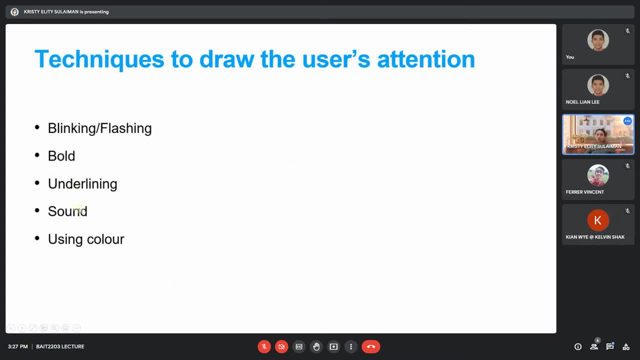 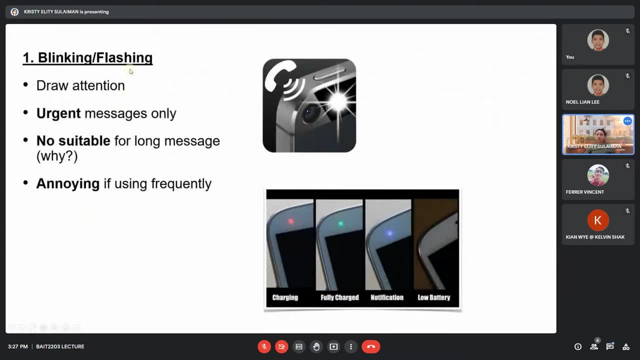 you can use bold, you can use underlining, you can use sound or you can use color in your ui design. so let's look at the first one, blinking and flashing. so usually this one is used to draw attention for urgent messages only. so previously, i think uh, ios, i'm not sure who started it here first. 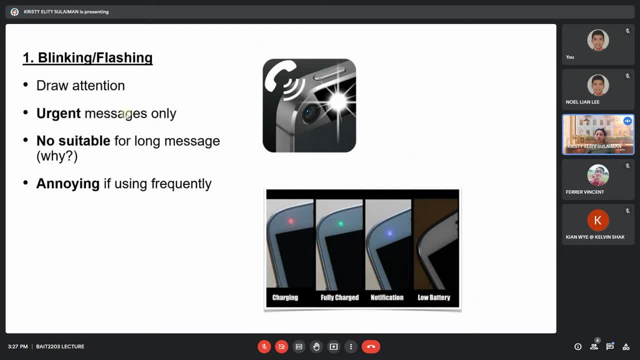 i think i, uh, but because i'm using ios, so i not. i know that this, this, this feature is enabled in ios. you can blink your flash if you got a call or you have a message right. so it is not suitable for, not suitable for long message, because it will be. 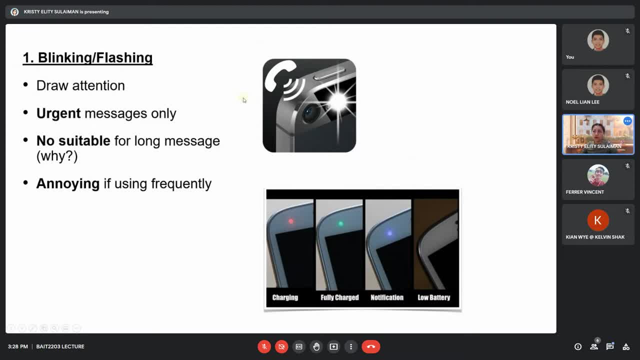 it will keep blinking and also for call okay, and it's annoying if using frequently, if it's used frequently, right. so like previously, when this um, this function was um, was introduced, like your, even, like my friend also using this blinking or flashing, flashing uh feature, like it's very irritating, like it's very annoying, like um, i'm cut. lovely from cold is cold, but 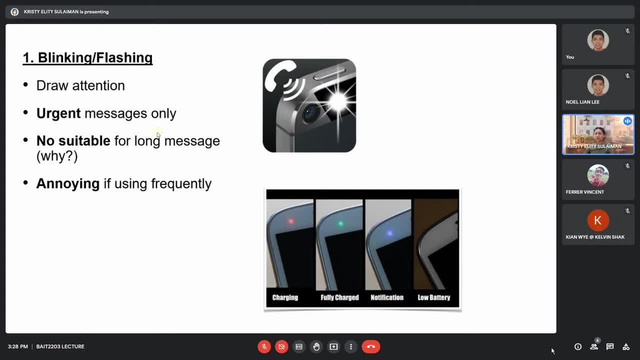 yeah, it's annoying. i don't think people prefer to use this anymore. maybe last time and also this one. also, you use this uh flashing to show that this the your subsystems, it's charging, it's red, fully charged is green and there is a notification: uh, blue and no battery. no, no. 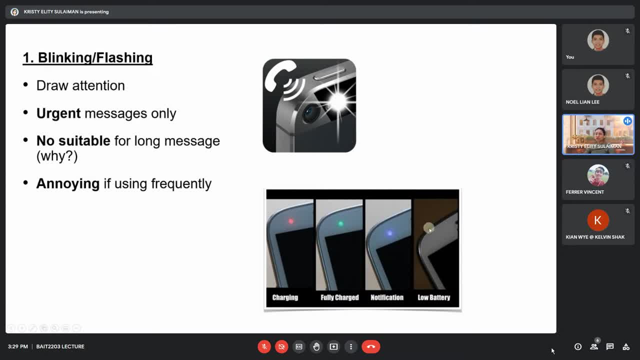 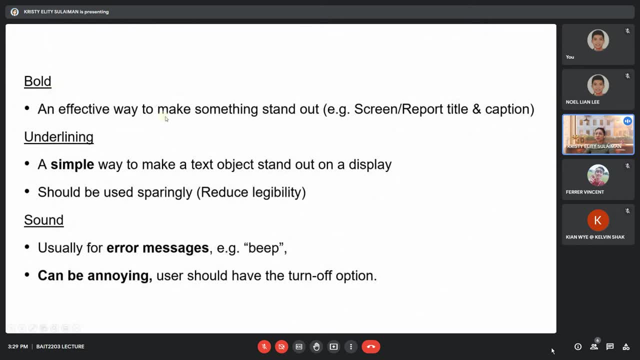 color icon. okay, so you can use this uh to design your ui, if it's applicable. and then you use bold. you want to make something stand out. uh, you can use this on screen report or title and caption or maybe like: if you do payment right, so you can pull your photo to pair and also underlining. 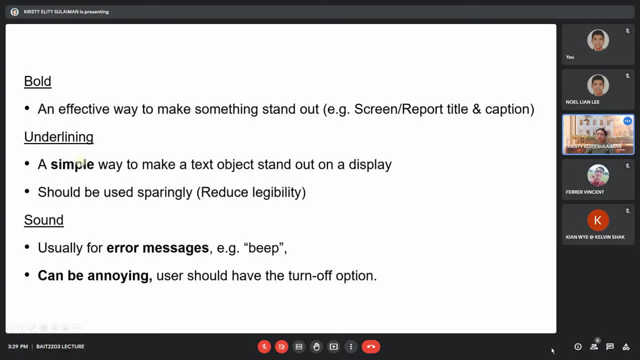 this is a simple way for you to make a text object stand out on a display, and you need to use this sparingly, not all the time, to reduce legibility of your ui design. and then you can also use sound. so sound in ui. usually you use them for error messages, like 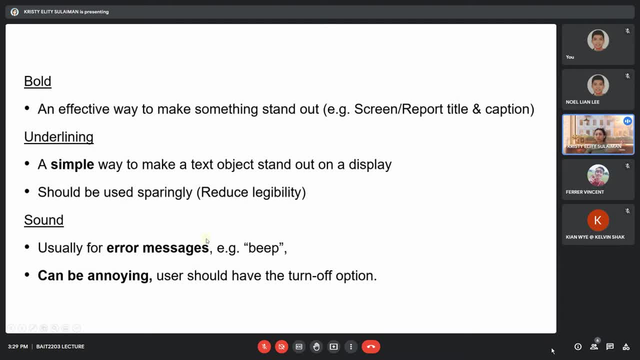 telling the user that something is wrong, but also, depending on the situation, like, um, if you like send email, if you send email like the sounds like whoosh demanded right, you have this kind of effect that's telling you that the email has been sent, and also every message like, if in windows it gives you something more, something like: 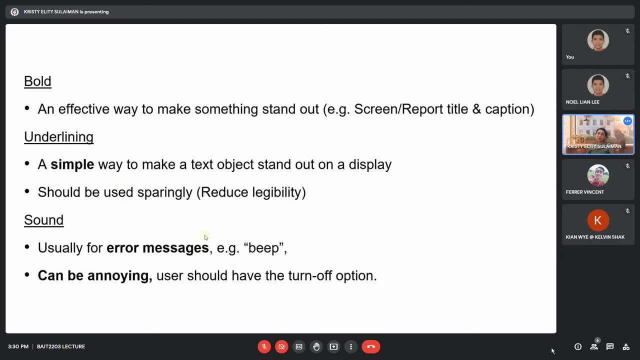 those are uh sound effects that um attract the user's attention. they can be annoying as well. so you can have, you can uh use if you like. if you want to enable this in your system, in your ui design, you need to also provide a turn off option. okay, so because 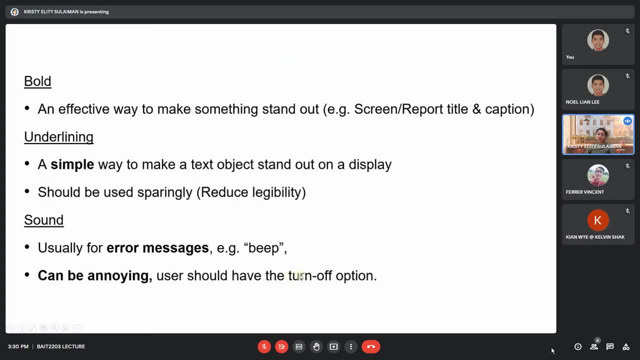 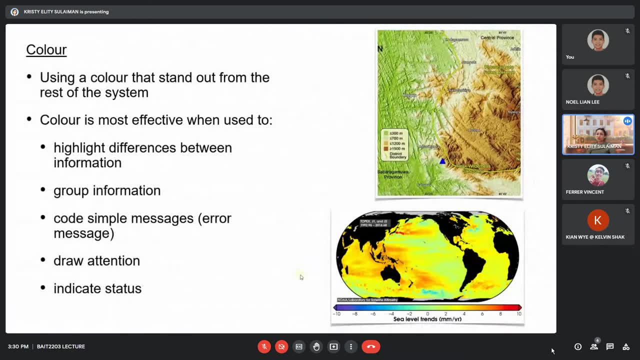 your user might not like it. so you can have the turn on option, okay, and then using colors: okay. so you use color that stand out from the rest of the system. so color is most effective for you to use when you want to highlight differences between information, like this one for, uh, sea level trends. this one um. 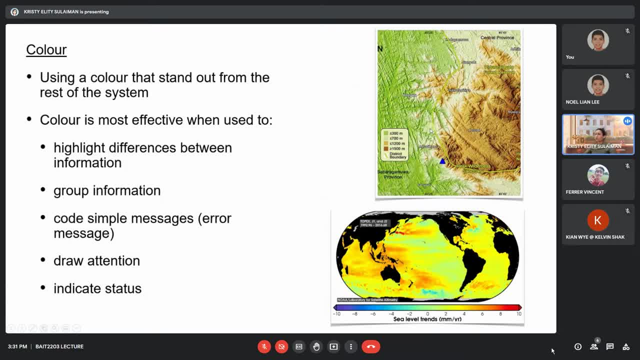 for a map of i'm not sure what is this um wind, this one. okay, so it shows. uh, it's used colors to show you the information. okay, so i also group information and also provide you with called simple messages, especially for error message. it can draw your attention. 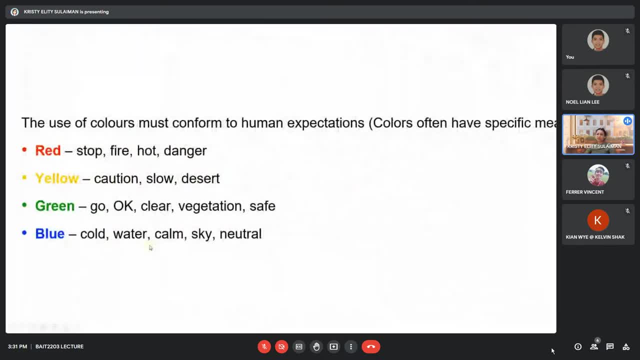 and it can indicate your, the status of your system. so the use of colors: it must confirm the human expectation. so color often have specific meanings depending on the culture getting. remember we had this class about culture last week, so red again. it's representing stop. it can be fire, maybe hot or danger. yellow. 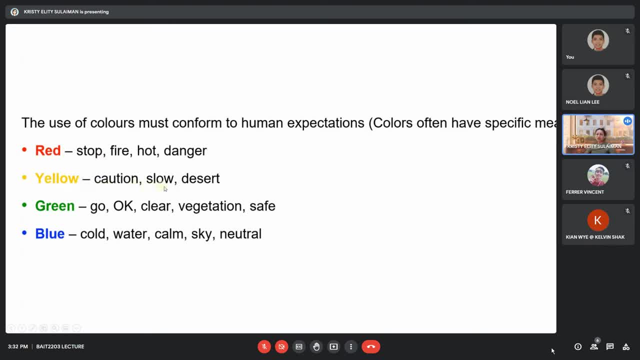 we use for caution, please go slow, or representing desert. green means go okay, it's clear vegetation and it's safe. blue indicates that it's cold, it's water, it's calm, it's high, it's neutral. so based on the user, your user capabilities or the user background, so you need to use the color according. 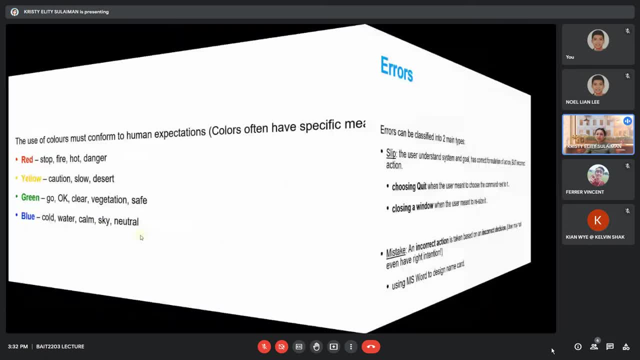 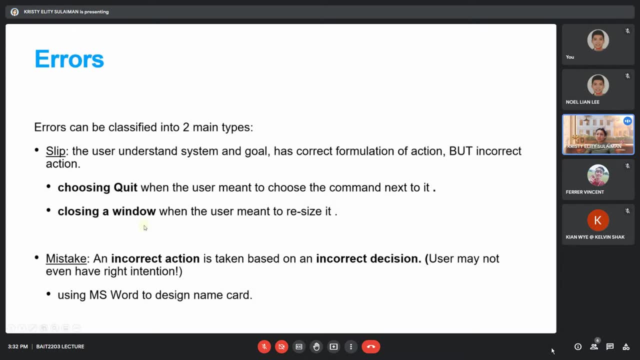 to their expectation. okay. next is errors. okay, so for errors we have two types. uh mean, these are the classification of errors in hci. for user design we have sleep and every stack, so sleep is sleep error. user understand the system goal and has correct formulation of action. okay, they already have. 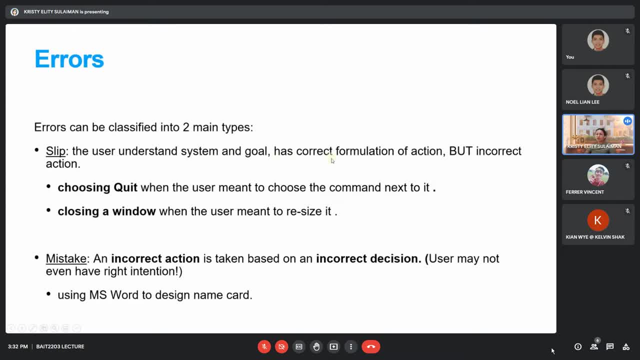 the goal, they understand the system, they already have the formulation of action, but they did incorrect action. okay, for example, like they choose quit when the user meant to choose the command next to it, like accidentally pick or click on quick button, and also another one is closing a. 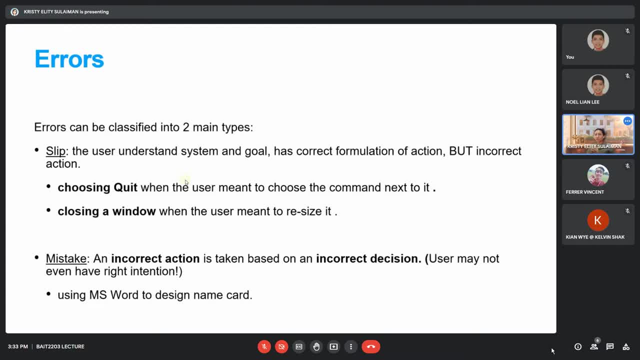 window when you were meant to resize it. yeah, yeah, and uh, that's for sleep, like, uh, it's like a mistake. uh, no, the mistake is another one. sleep is that when you, you already know what to do, but you, you did an incorrect action. okay, you meant to close the window, but 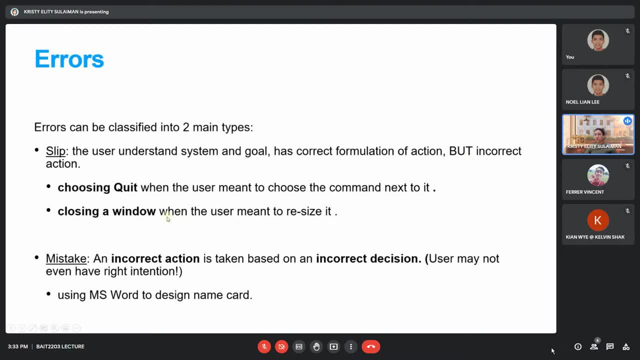 you meant to resize the window, but you then pick to close the window. okay, another type of error. we have mistake, so this is an incorrect action that is taken based on incorrect decision from the beginning. you already have incorrect decision. like you don't have the right intention for you to proceed with your goal. okay, 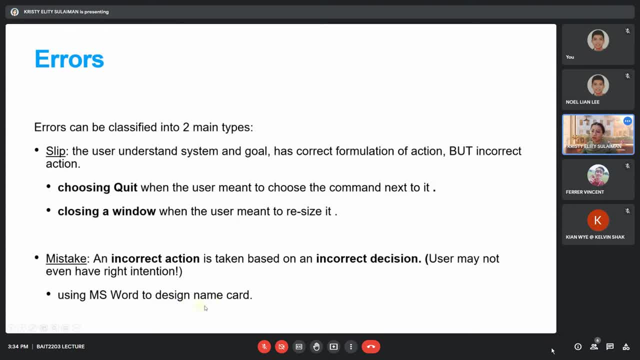 so your goal here is to design a name card. okay, so you design a name card using my microsoft void, so so forth. is um with word processing? it's not for designing, we know we can do that, but um, in this case um, you are using a wrong, wrong software to design a name card. you should, you can use, maybe. 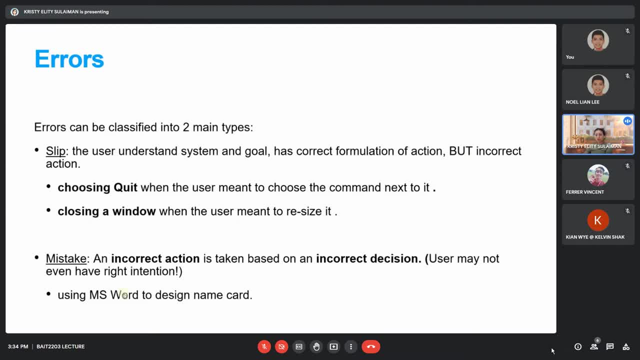 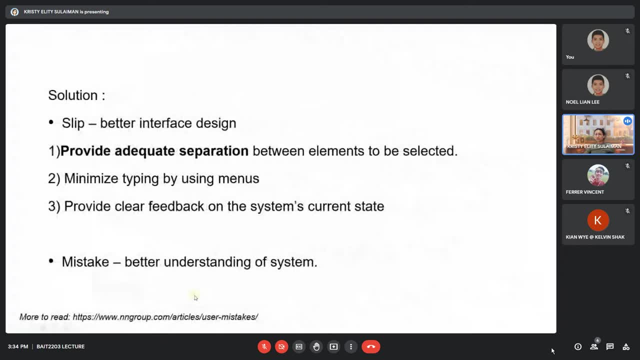 um, we have illustrator, we have photoshop, we have other software that is intended for designing name. okay, so we have solution for these areas for sleep. you need to have a better interface design, so here you can provide adequate separation between your elements like your button, your x button and also your resize button. you provide adequate um separation. 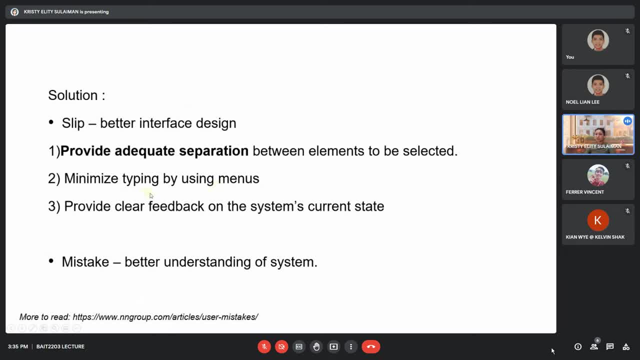 gap between them and you minimize typing by using menus, trying to use menus, and you provide clear feedback on the system's current state. okay, so that they usually know what to do next. and then you stack. usually usually: um, how do we, how do you tackle this? you need to have a better understanding of a system if it's uh, you want to use. 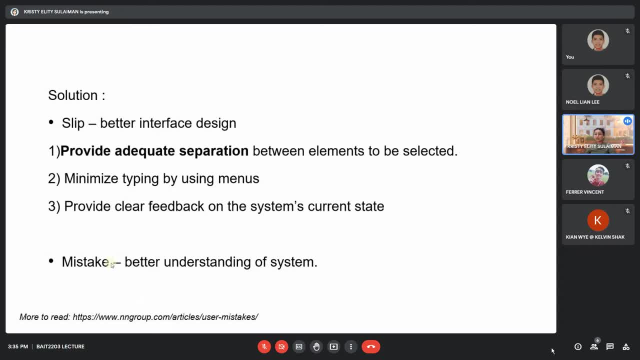 you want to use like powerpoint to design a name card, it's not wrong, okay. but in terms of hci, the system powerpoint is for our points, like right for presentation, it's not for designing, okay. so that's why, um, if you refer back to the system and you go back to your goal, what you want, 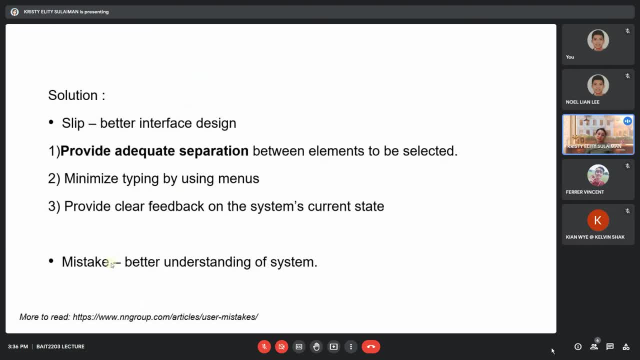 to do, but of course you still can design name card using whichever whatever tools that you have. like word, also, you can use it to design your name, but there's no problem, actually. okay, but uh, for this idea. it's just giving you an idea on how you should. you need to understand the use of the. 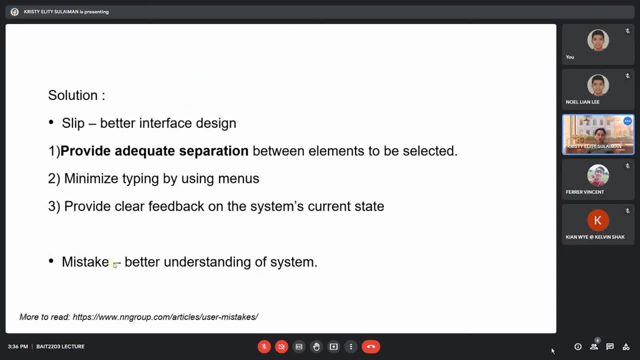 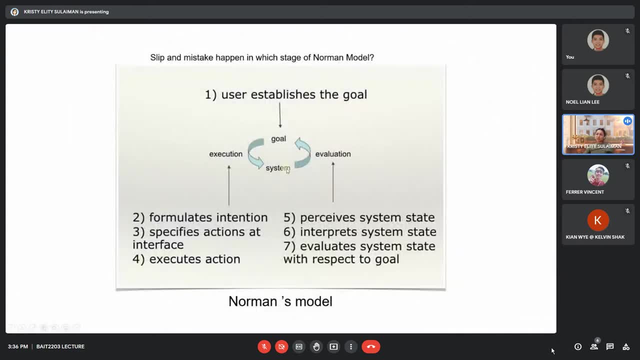 system when you want to achieve your goal. okay, so in this, uh, in this normal model, where does this sleep and mistake happen? okay, so it can happen in when you formulate intention. okay, it can happen when you formulate intention like, um the sleep you form already formulate the intention and then, um, you specify the actions at the interface. but 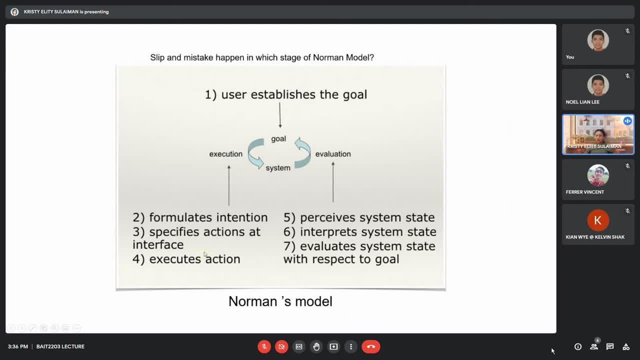 you execute wrongly. okay for mistake. definitely from formulating intention. you have the goal to design the card, the name card, but you give you, you, uh, you do mistakes when you formulate your intention, like what software you want to use? okay, so for sleep is, when you execute action, you already have a correct intention, you already have a specified. 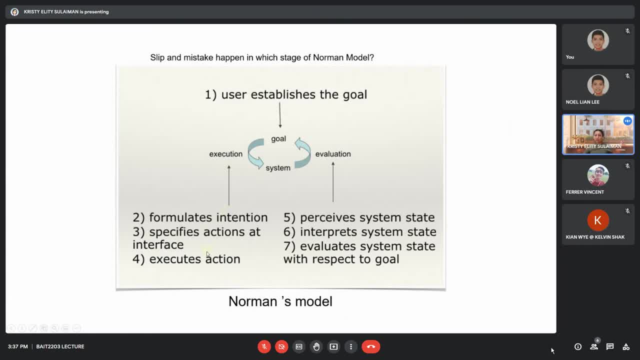 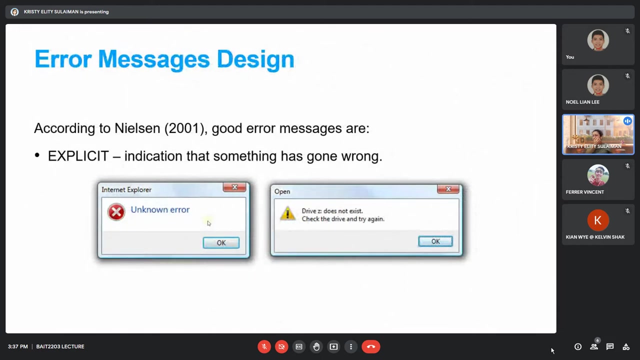 action for the interface that you already know where to go, but when you execute the action, you make a mistake. you did an error, okay, so sleep happened at stage four, while mistake happened at stage two, and then we have this error messages beside. so, um, according to this- uh, this researcher- good error messages are explicit. okay means you. 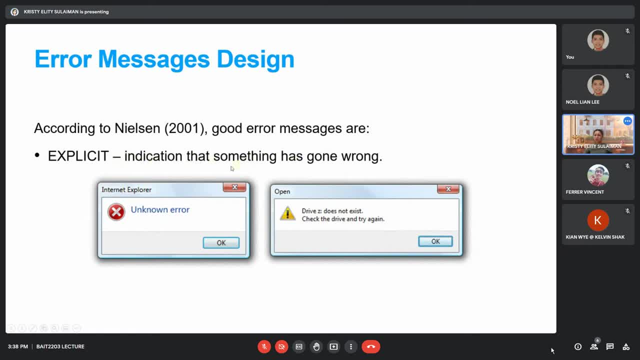 indicate that something has gone wrong. right, so your error message design should tell the user what to do next and what is the error of all. okay, like for this one, this is not helpful at all. right, i haven't. you have an unknown error, so what should i do next? and i click okay. 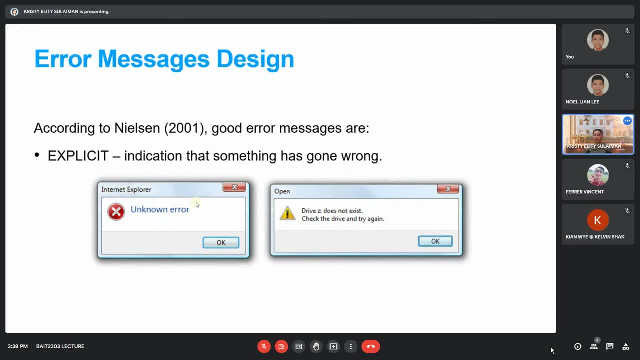 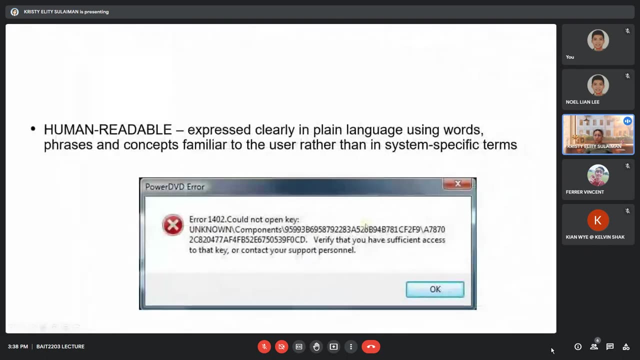 and i get the error again. so you don't know how to go from there. and unlike this one. so it tells you that this drive z does not exist and it gives you the solution. you check the drive and try again. okay, and also it should be human readable. your error should be human readable, which is expressed. 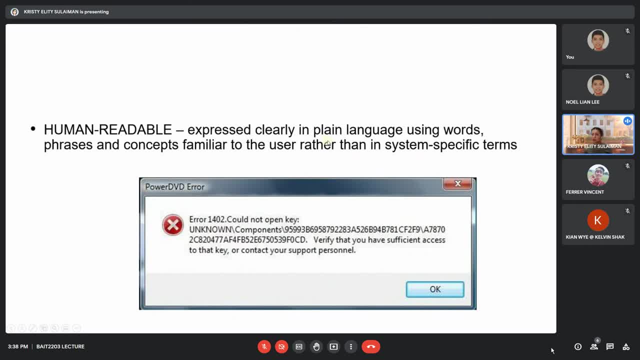 clearly in plain language, using words right and uses phrases and concepts familiar to the user, then in system specific terms like this: okay, so this is like more to like technical terms, like putting up on the key. what case is, and then, very kind, that you have sufficient access to that. 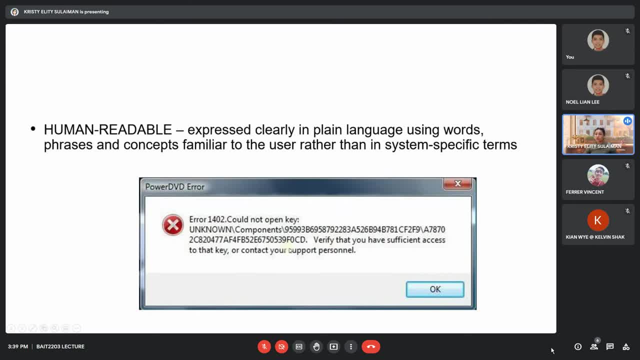 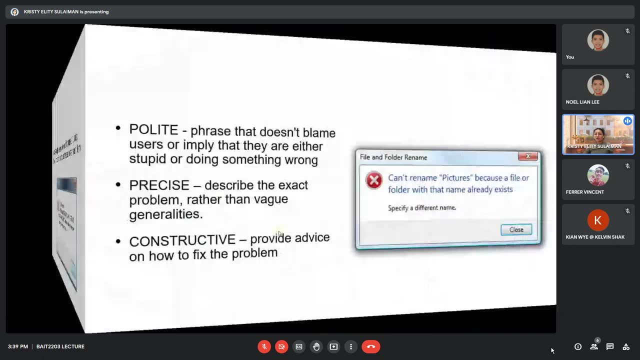 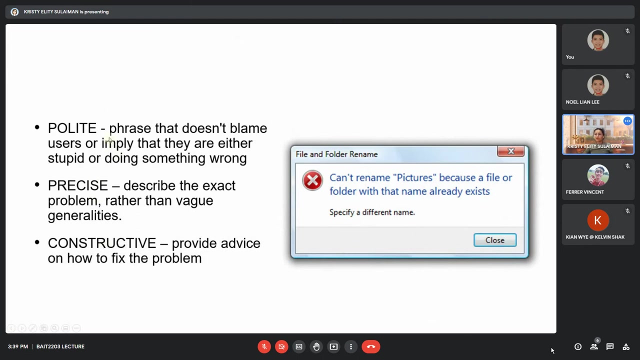 key or compare your skill personnel, and then you also don't know who is your support personnel, right? so you, you need, you need to provide an error message that is clear to the user, and then what to do next about the error. your error also should be polite, okay. should be precise and constructive, okay. so when you 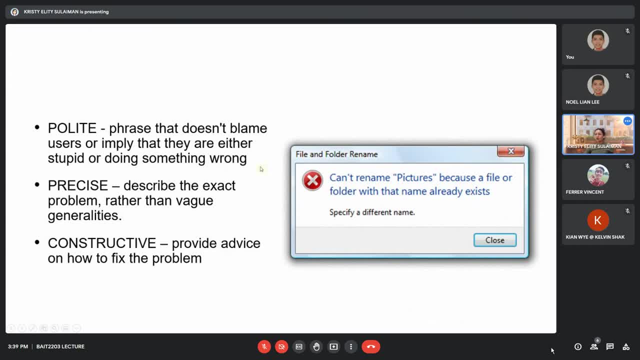 when you design your error message, you use phrase that does not blame the user or imply that they are either stupid or doing something wrong. you just like. you just be polite. like you cannot do this, okay, i like this one. you cannot rename the pictures, okay before. like it's not. you cannot say: 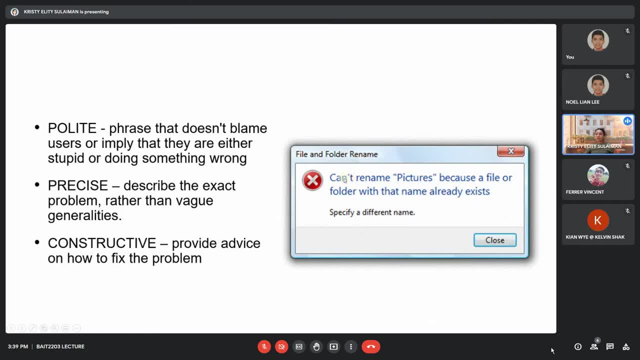 like you made those, you made the stupid, you made a stupid uh rename, you made a stupid dream. okay, maybe you, if you do that, like that the user will like. of course the user will be like: taken aback, right. and then you need to be precise. you describe the exact problem like you tell the user that 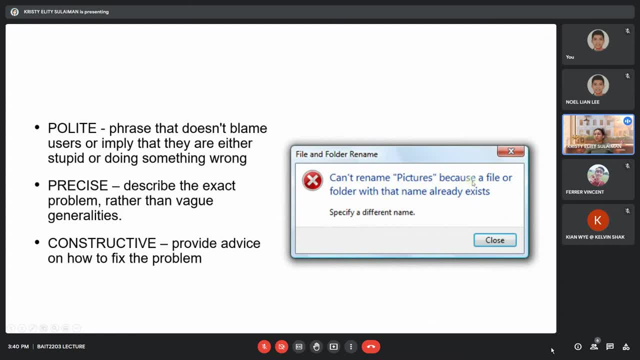 you cannot rename the picture because there is another file that has the same, select the same name, and then you give a constructive, um, constructive advice, like you give a solution on how to fix the problem so you can specify a different name. okay, so these are how, how you can um. 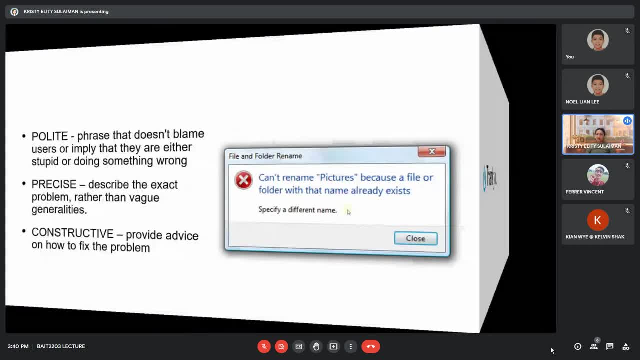 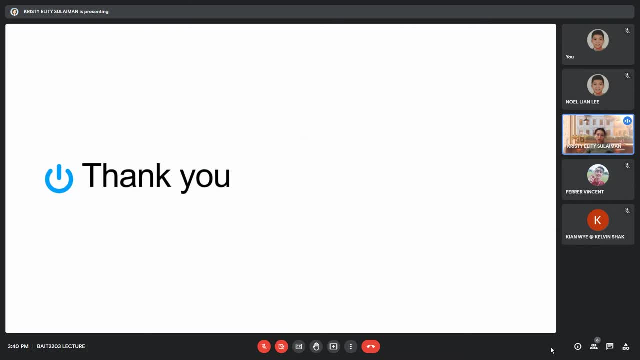 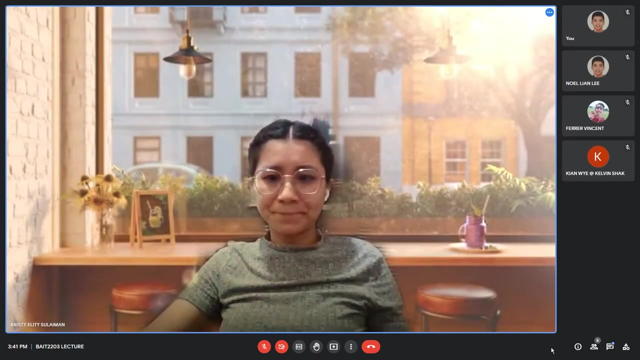 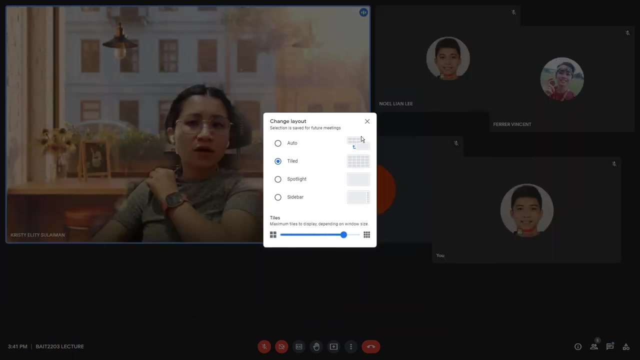 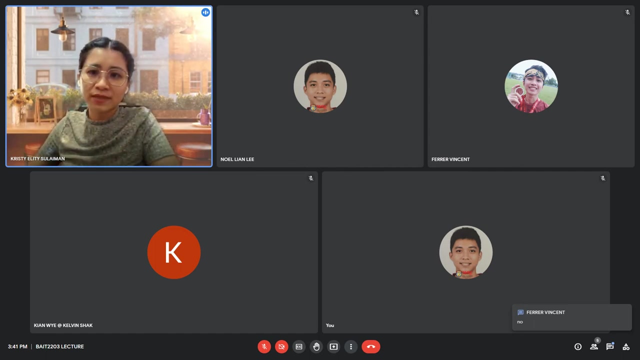 design your error messages. okay, so that's all for today's lecture. i hope you all gain new knowledge and i hope you can apply the knowledge that you learned today to your ui design. any question, i don't, they're okay, no question. so okay, okay, so, so i want you all to continue doing your assignment. we are already in week six, so 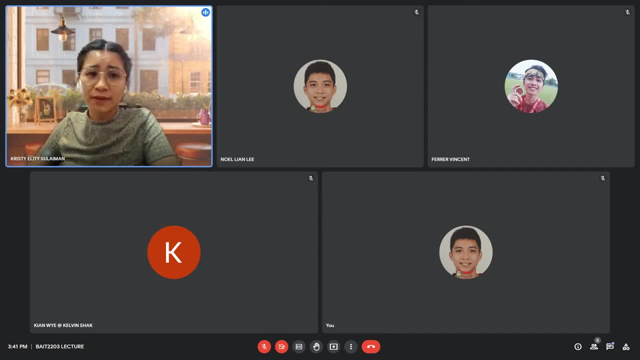 you should have. you should make progress for your assignment so that you don't um have last minute work, okay, so if you have no more questions and if you go do your things now, but you only left the session mid session at 3: 50.. can you do that okay? 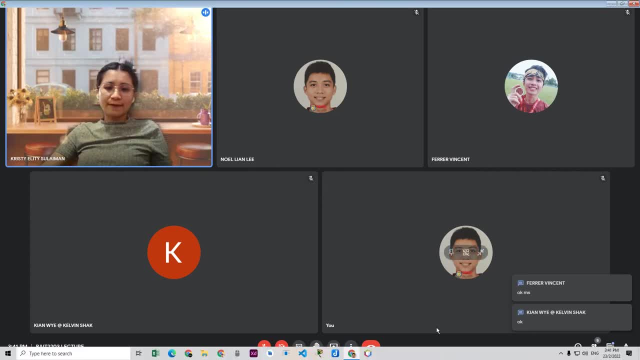 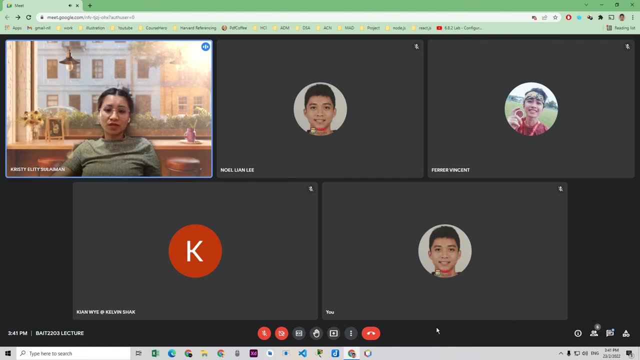 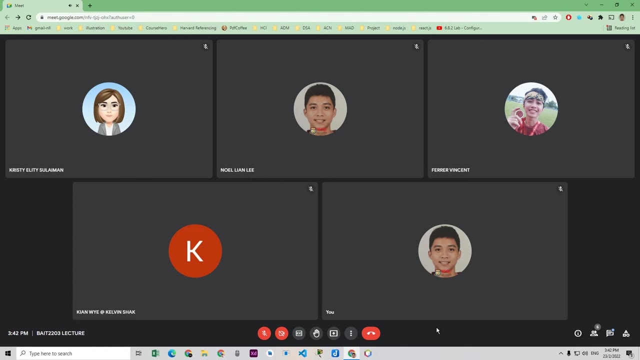